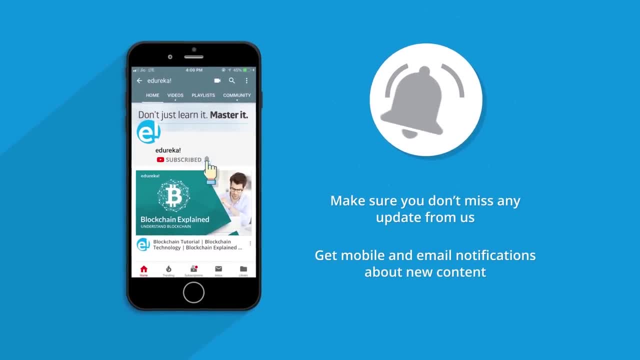 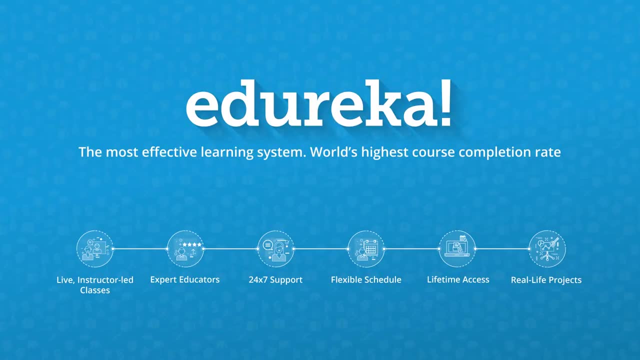 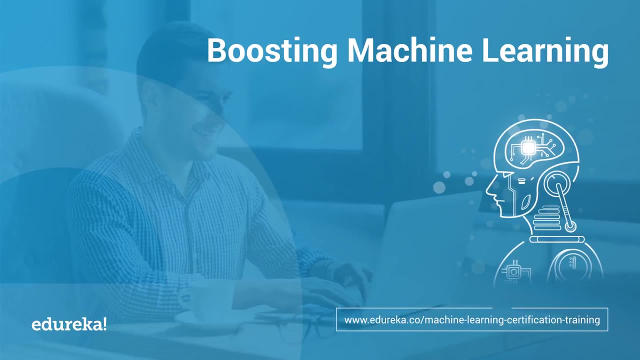 Since we're generating an immeasurable amount of data, It has become a need to develop more advanced and complex machine learning techniques. boosting machine learning is one such technique that can be used to solve complex data-driven real-world problems. Hi everyone, I'm Zulekha from Edureka. 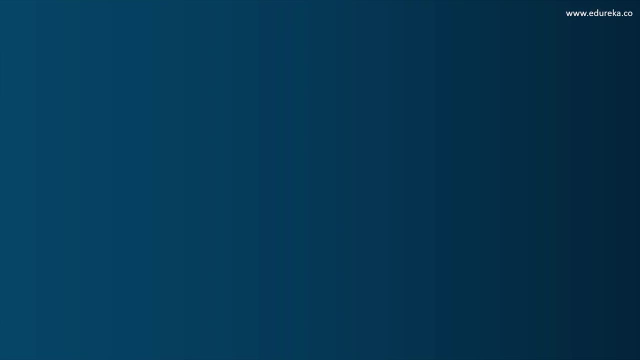 and I welcome you to this session on boosting machine learning. Let me quickly run you through today's agenda. We're going to begin the session by understanding why boosting is used. after that We'll understand what exactly boosting means in machine learning, will move on. 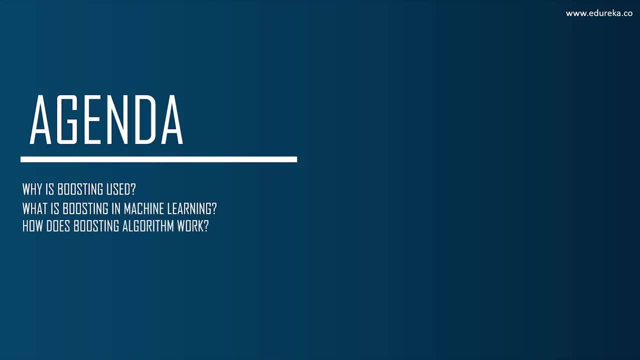 and discuss how the boosting algorithm works, and we'll finally discuss the different types of boosting, which include adaptive boosting, gradient boosting and XG boost. We finally end the session by looking at a practical implementation in python, where we'll understand how boosting machine learning algorithms can be used. 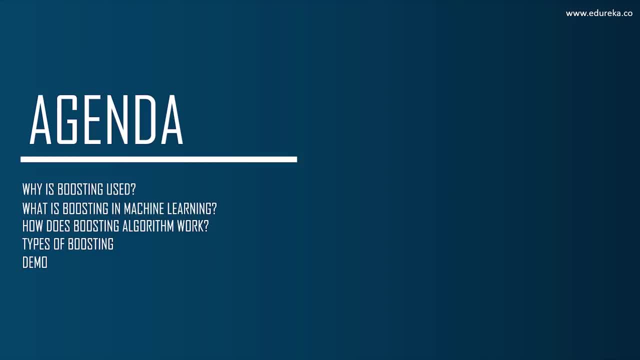 to improve the accuracy of a model. So, guys, before I move any further, make sure that you subscribe to Edureka YouTube channel in order to stay updated about the most trending technologies. Now let's take a look at our first topic. So why exactly are we using boosting machine? 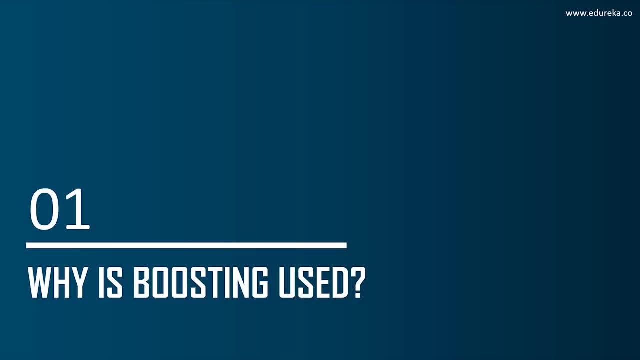 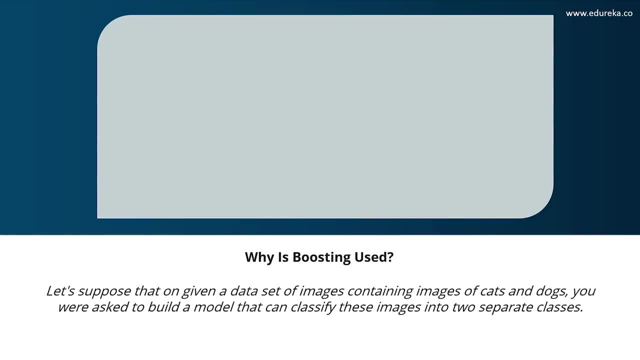 learning techniques. before I tell you what it is, Let's understand what led to the need of boosting machine learning. in order to solve complex and convoluted problems, We require more advanced techniques Right now. let's suppose that, given a data set of images containing cats and dogs, 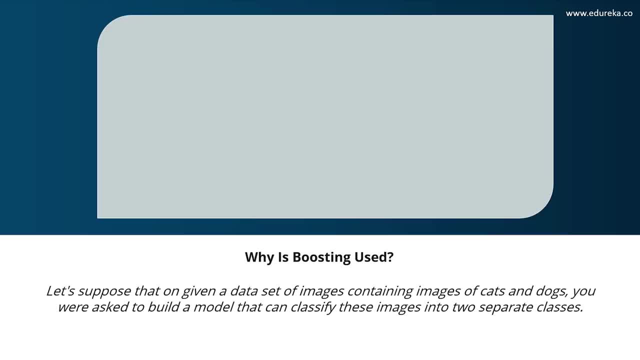 You are asked to build a machine learning model that can classify these images into two separate classes. Now, like every other person, you will start by identifying the images by using some rules. Let's say, the image has pointy years is a rule. Now, if the image has pointy years? 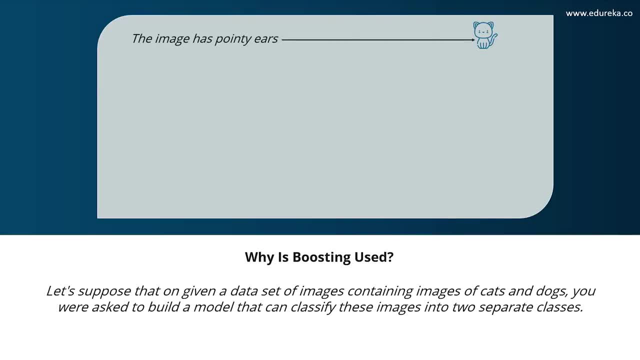 then it's a cat, right? similarly, let's say, you've created another rule, which is the image has cat shaped eyes, which means it's a cat Again. now, if the image has bigger limbs, and then it's a dog, and if the image has sharpened claws. 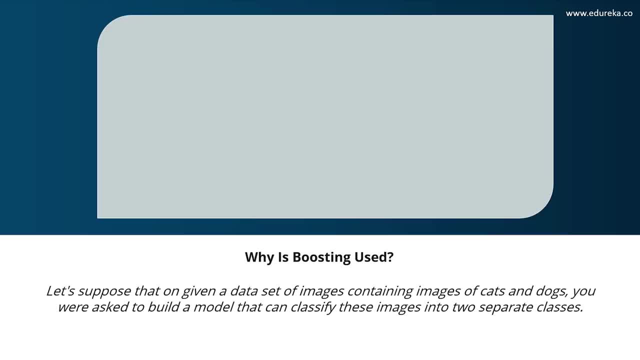 You are asked to build a machine learning model that can classify these images into two separate classes. Now, like every other person, you will start by identifying the images by using some rules. Let's say, the image has pointy years is a rule. Now, if the image has pointy years? 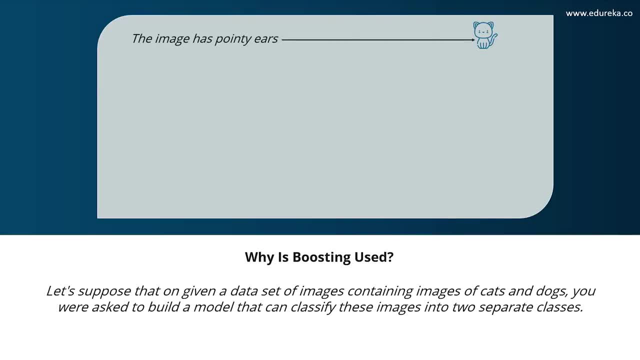 then it's a cat, right? similarly, Let's say, you've created another rule, which is the image has cat shaped eyes, which means it's a cat. Again. now, if the image has bigger limbs, and then it's a dog, and if the image has sharpened claws. 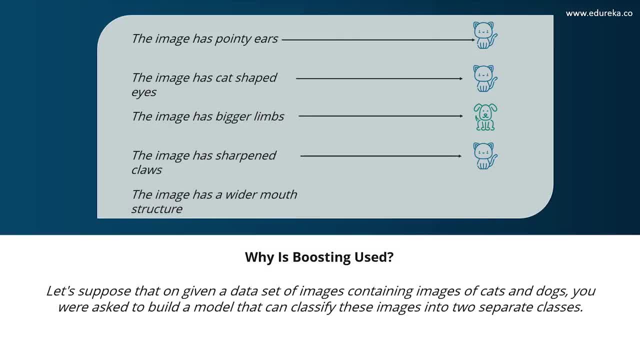 then it's a cat. Similarly, if the image has a wider mouth structure, then it's a dog. right now, These are some rules that we define in order to identify whether it is a cat or a dog, using one of these rules to classify the image. 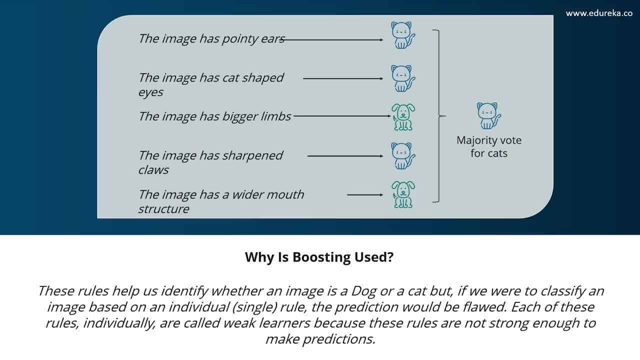 It does not make sense. Okay, let's say that the cat is of a different breed and it has bigger limbs, and you give an input image and the rule says: the image has bigger limbs, It'll classify it as dog. Now, each of these rules, if applied individually on an image, 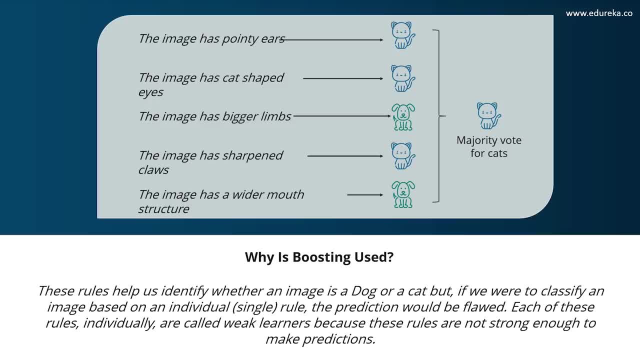 will not give you an accurate result. Right, you'll have to apply all of these rules and make sure that image goes through all these rules and only then predict the output. So each of these rules individually are called weak learners, because these rules are not strong enough. 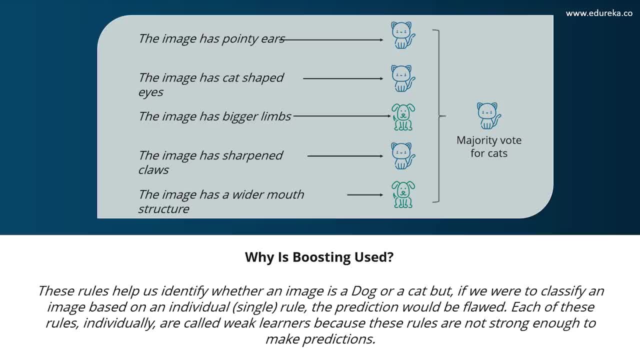 to classify an image as a cat or a dog individually. Okay, what I'm saying is, if you just use one rule to classify an image as a cat or a dog, then your prediction will mostly be wrong. You cannot take one feature into consideration. 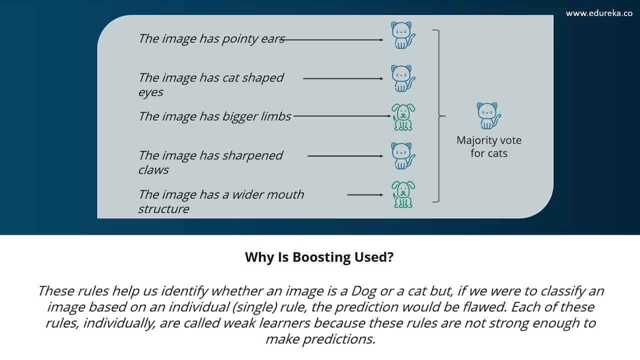 and classify the images either cat or dog. So to make sure that our prediction is more accurate, we can combine the predictions from each of these weak learners by using the majority rule or weighted average Right. this is exactly what a strong learner model is. 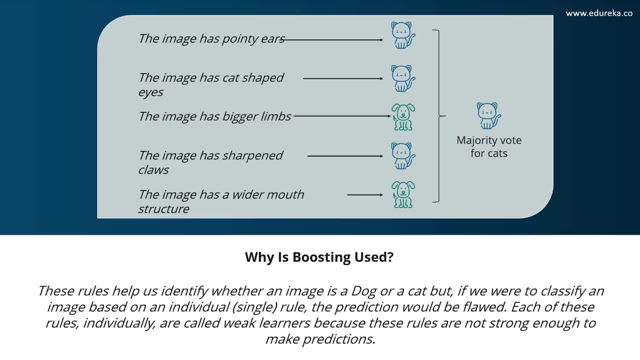 So in the above example, what we did is we've defined five weak learners, and the majority of these rules give us a prediction that the image is a cat. That's why our final output is a cat. Right here you can see that three of these rules classify: 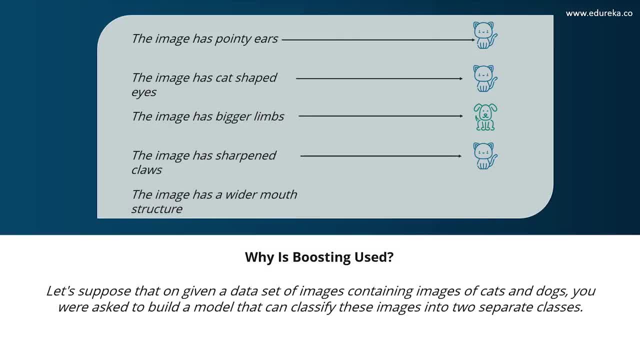 then it's a cat. Similarly, if the image has a wider mouth structure, then it's a dog. right now, These are some rules that we define in order to identify whether it is a cat or a dog, using one of these rules to classify the image. 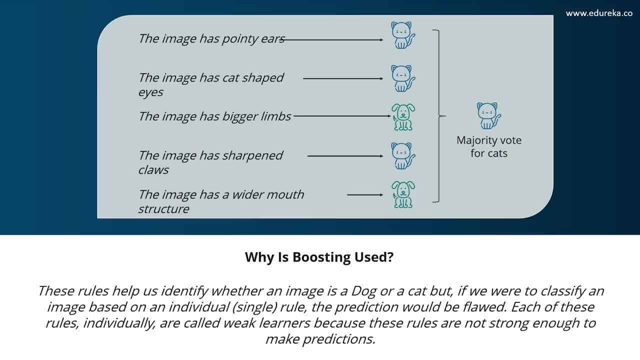 It does not make sense. Okay, let's say that the cat is of a different breed and it has bigger limbs, and you give an input image and the rule says: the image has bigger limbs, It'll classify it as dog. Now, each of these rules, if applied individually on an image, 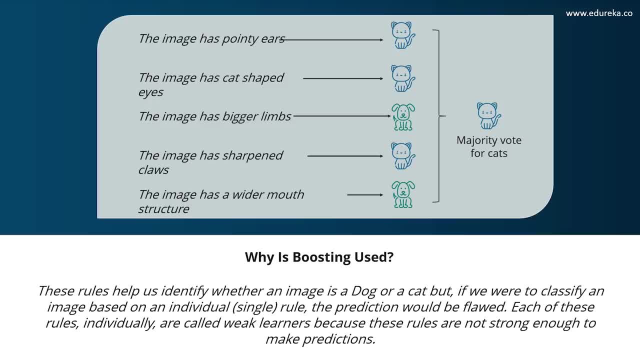 will not give you an accurate result. Right, you will have to apply all of these rules and make sure that image goes through all these rules and only then predict the output. So each of these rules individually are called weak learners, because these rules are not strong enough. 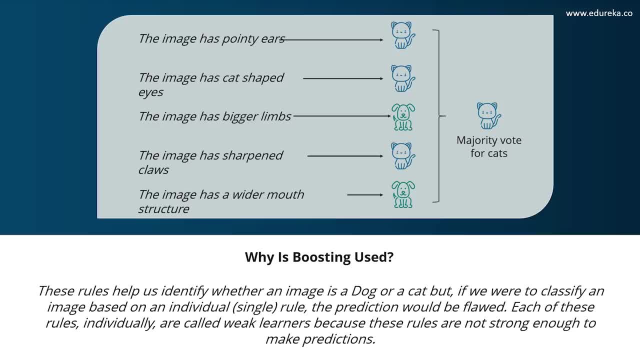 to classify an image as a cat or a dog individually. Okay, what I'm saying is, if you just use one rule to classify an image as a cat or a dog, then your prediction will mostly be wrong. You cannot take one feature into consideration. 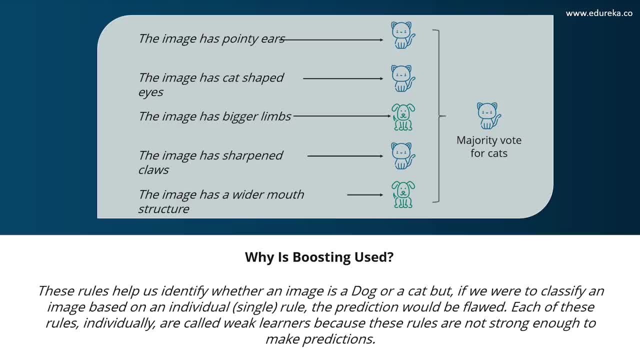 and classify the images either cat or dog. So to make sure that our prediction is more accurate, we can combine the predictions from each of these weak learners by using the majority rule or weighted average right. This is exactly what a strong learner model is. 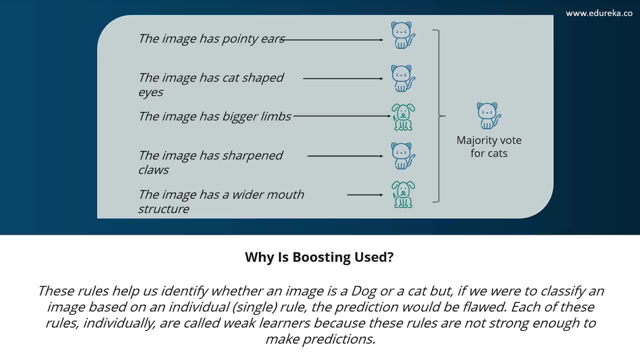 So in the above example, what we did is we've defined five weak learners, and the majority of these rules give us a prediction that the image is a cat. That's why our final output is a cat. right here You can see that three of these rules classify the image. 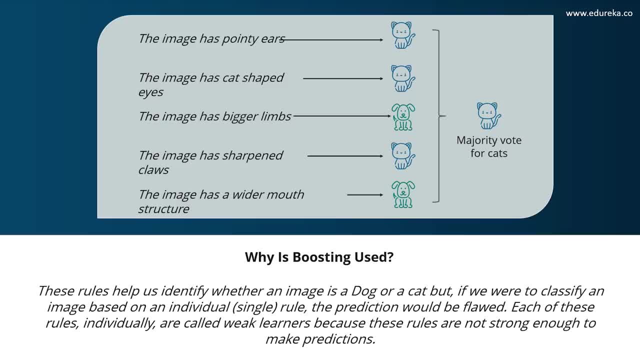 as a cat and two of them classify it as a dog, So our majority says that this is a cat, So we're going to go with cat. This is what a strong learner module is. It'll just combine all the weak learners in order to give you a more precise 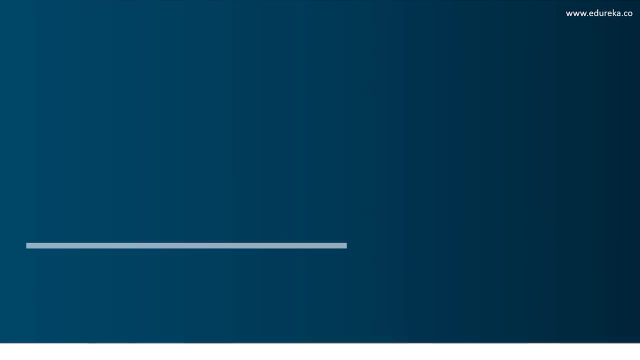 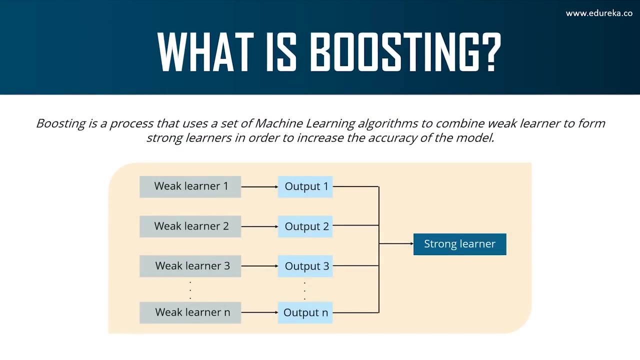 and a more accurate prediction. Now this brings us to the question: What exactly is boosting? Boosting is an ensemble learning technique that uses a set of machine learning algorithms in order to convert or combine weak learners to strong learners, in order to increase the accuracy of the model. 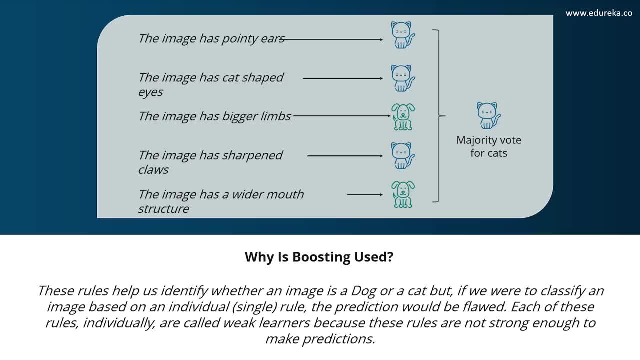 the image as a cat and two of them classify it as a dog. So our majority says that this is a cat, so we're going to go with cat. This is what a strong learner module is. It'll just combine all the weak learners. 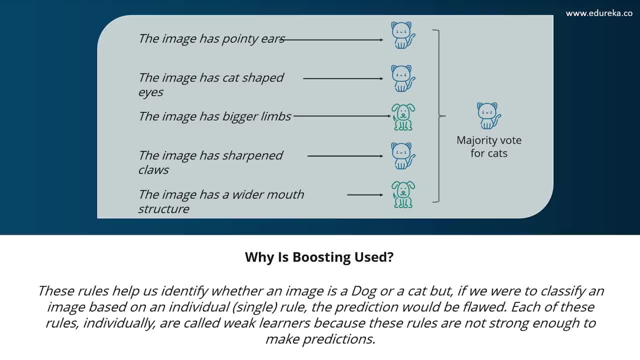 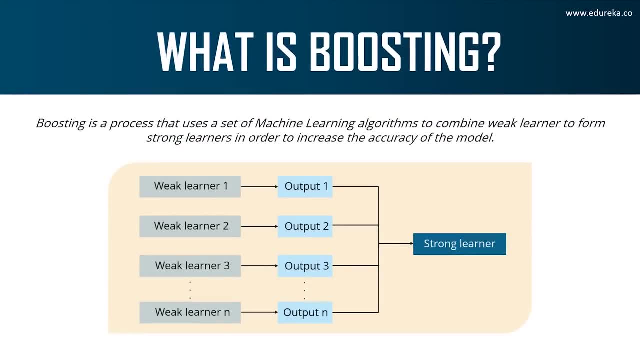 in order to give you a more precise and a more accurate prediction. Now this brings us to the question: what exactly is boosting? Boosting is an ensemble learning technique that uses a set of machine learning algorithms in order to convert or combine weak learners to strong learners, in order 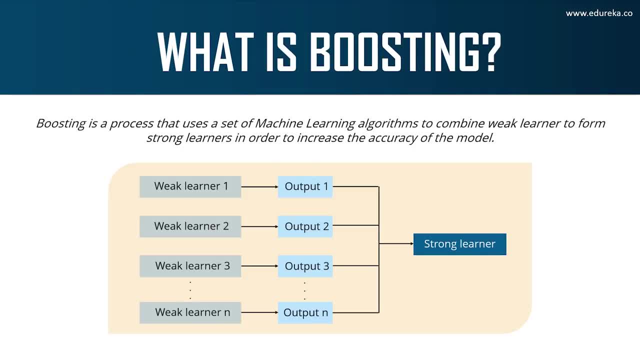 to increase the accuracy of the model. So, guys, boosting is actually a very effective method in order to increase the efficiency of your model. In most of these competitions that you see on Kaggle or any machine learning competition, maximum of the competitors- or, you know, the winners- usually implement boosting. 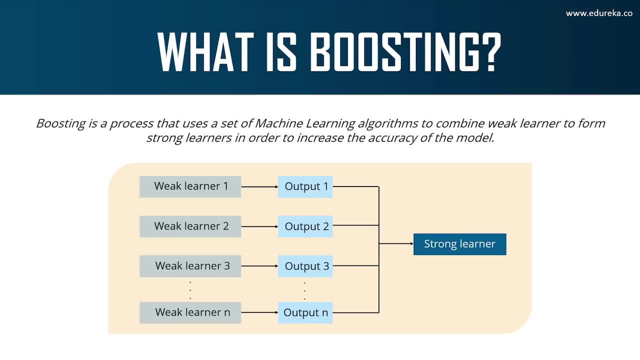 and bagging or any other ensemble learning technique. Now, for those of you who don't know what ensemble learning is, don't worry, I'll be covering that in the next slide. So, as you can see from the figure, we're combining the outputs or the predictions. 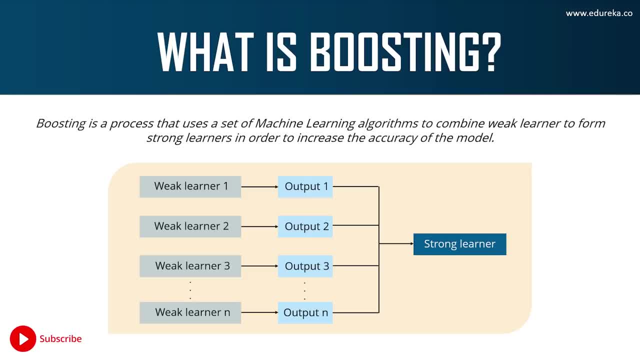 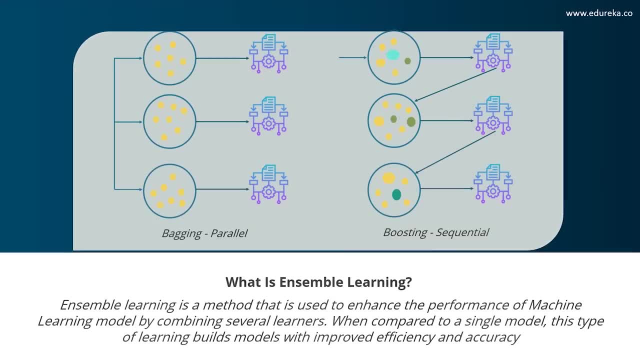 that we get from all our weak learners or our rules, in order to get a strong learner right. So this is the basic principle behind boosting. Now let's understand what ensemble learning is. Ensemble learning is basically a technique that is used to enhance your model performance. 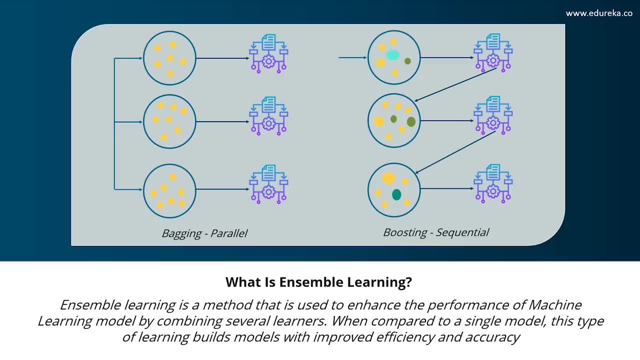 and its accuracy. This is exactly why ensemble methods are used to win market-leading competitions such as the Netflix recommendation competition and other Kaggle competitions. right So, maximum of your winners will always be implementing ensemble learning models. So under ensemble learning, we have two types. 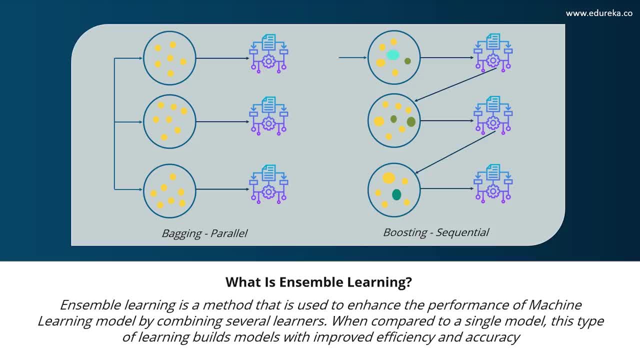 We have sequential ensemble and parallel ensemble. So, guys, before you get confused, let me tell you that boosting is a type of ensemble learning. boosting and bagging are the two different types in which you can perform ensemble learning. So the first type of model is the sequential ensemble model. 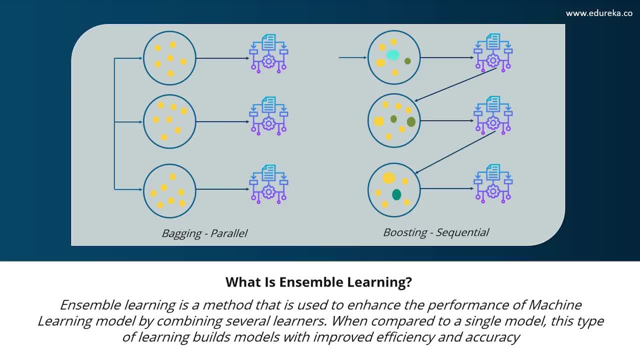 which is popularly known as boosting. here The weak learners are sequentially produced during the training phase. The performance of the model is improved by assigning a higher weightage to the previous incorrectly classified samples. An example of boosting is the adaptive boosting algorithm. Now in boosting ensemble learning. 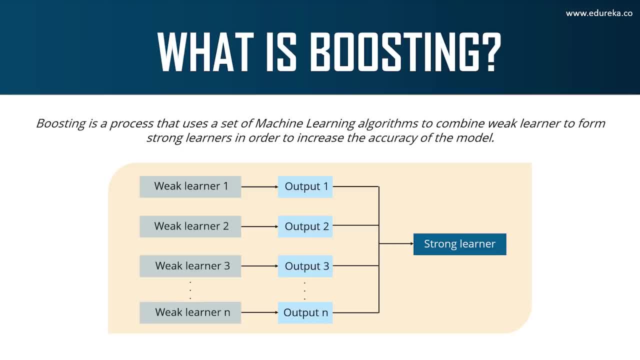 So, guys, boosting is actually a very effective method in order to increase the efficiency of your model. in most of these competitions that you see on Kaggle or any machine learning competition, maximum of the computers or you know, the winners usually implement boosting and bagging or any other ensemble learning technique. 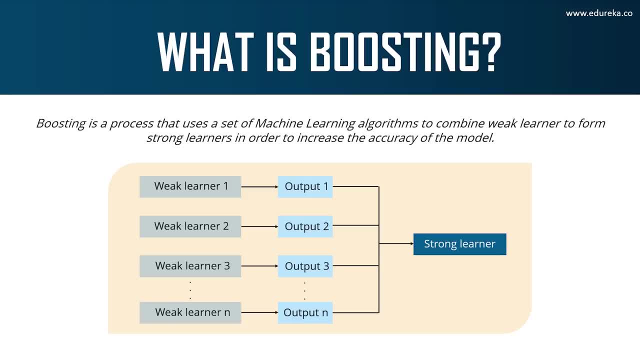 for those of you who don't know what ensemble learning is, Don't worry, I'll be covering that in the next slide. So, as you can see from the figure, we're combining the outputs or the predictions that we get from all our weak learners. 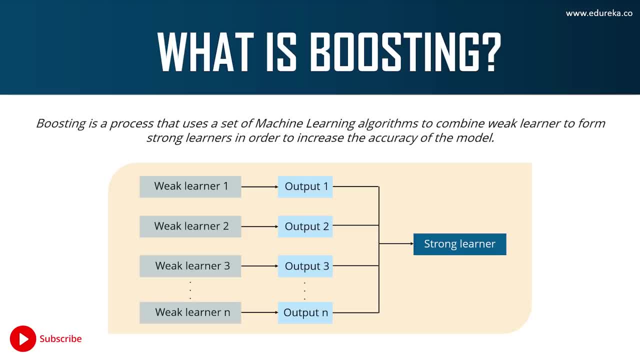 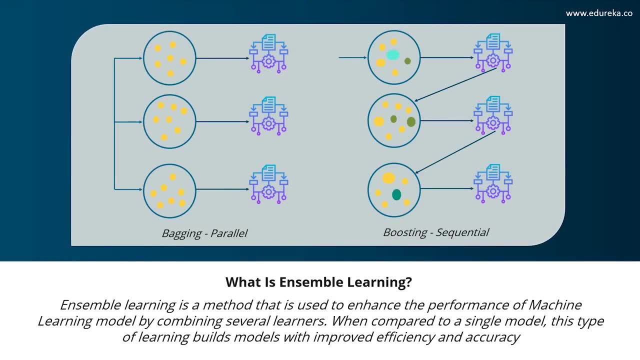 or our rules in order to get a strong learner right. So this is the basic principle behind boosting. now let's understand what ensemble learning is, and simple learning is basically a technique that is used to enhance your model performance and its accuracy. This is exactly why ensemble methods are used. 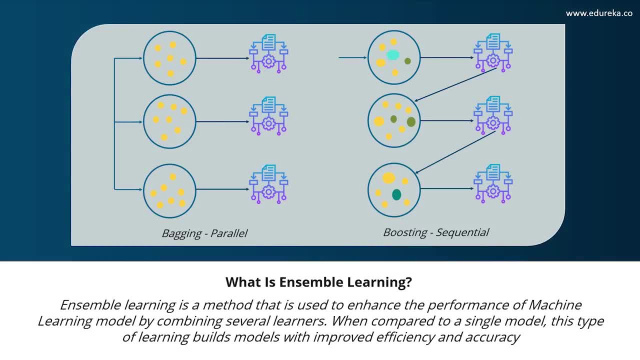 to win market leading competitions, such as the Netflix recommendation competition and other Kaggle competitions right to maximum of your winners will always be implementing ensemble learning models. So under ensemble learning, we have two types. We have sequential ensemble and parallel ensemble. So, guys, before you get confused, 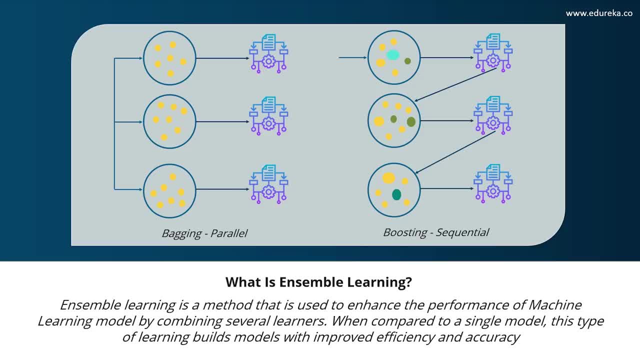 let me tell you that boosting is a type of ensemble learning. boosting and bagging are the two different types in which you can perform ensemble learning. So the first type of model is the sequential ensemble model, which is popularly known as boosting. here The weak learners are sequentially produced. 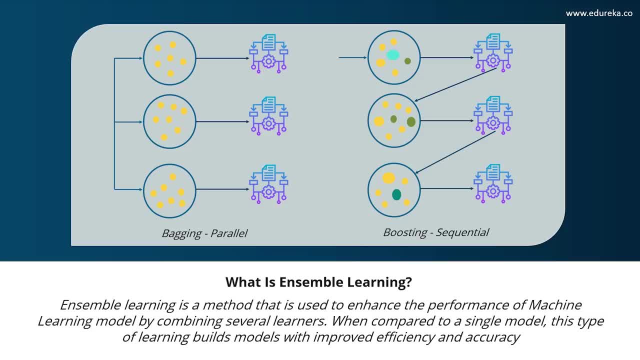 during the training phase, the performance of the model is improved by assigning a higher weightage to the previous incorrectly classified samples. an example of boosting is the adaptive boosting algorithm. now, in boosting ensemble learning, what happens is you feed your entire data set to your algorithm and the algorithm will make some predictions. 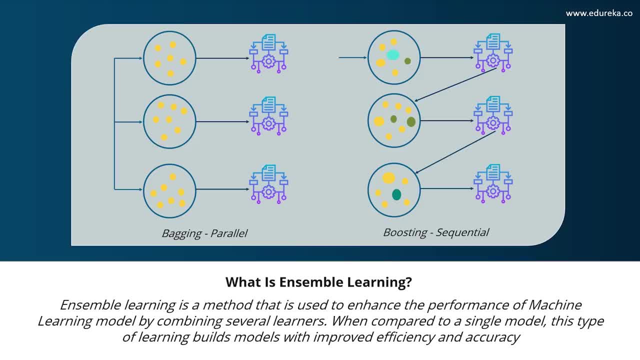 Let's say, the algorithm misclassified some of your data. Now what happens in boosting is you pay more attention to the misclassified data points, you increase our weightage and therefore you make it a point that a lot more importance is given to these misclassified values. 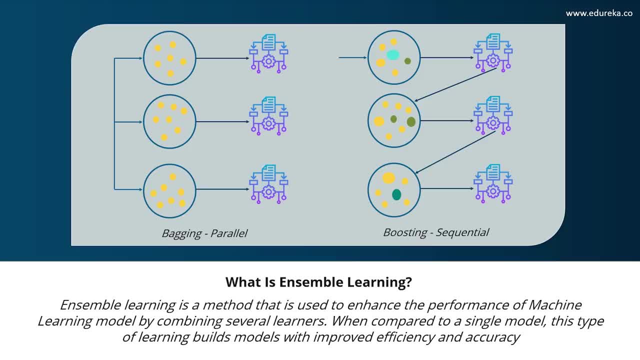 You keep doing this until all your wrongfully predicted or your misclassified samples are correctly predicted. right, That's how you increase the efficiency of your model. Then we have something known as parallel ensemble learning, also known as bagging. here The weak learners are produced parallelly. 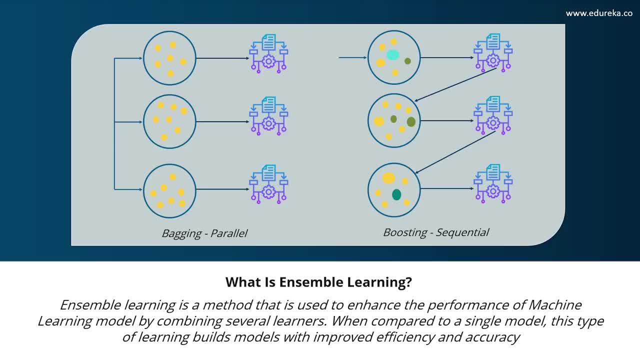 what happens is you feed your entire data set to your algorithm and the algorithm will make some predictions. Let's say the algorithm misclassified some of your data. Now what happens in boosting is you pay more attention to the misclassified data points. You increase our weightage. 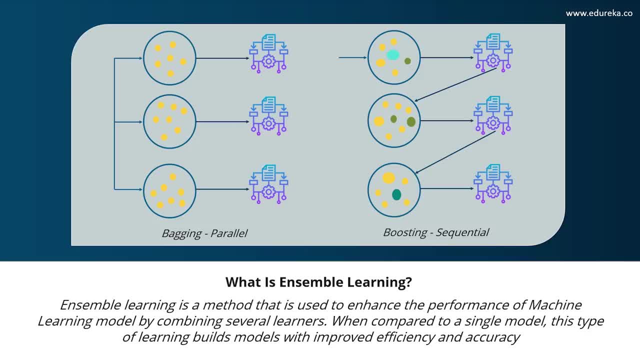 and therefore you make it a point that a lot more importance is given to these misclassified values. You keep doing this until all your wrongfully predicted or your misclassified samples are correctly predicted. Right, that's how you increase the efficiency of your model. 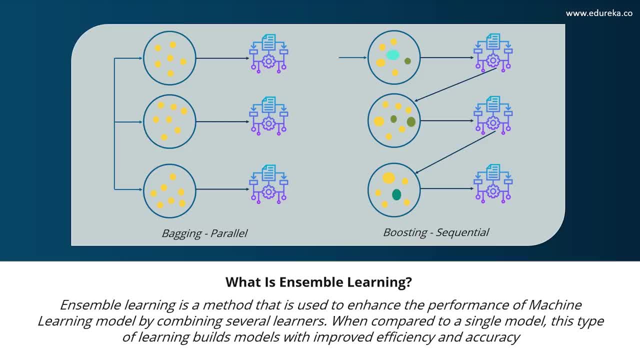 Then we have something known as parallel ensemble learning, also known as bagging. Here the weak learners are produced parallelly during the training phase. Now the performance of the model can be increased by parallelly training a number of weak learners on a bootstrapped data set. 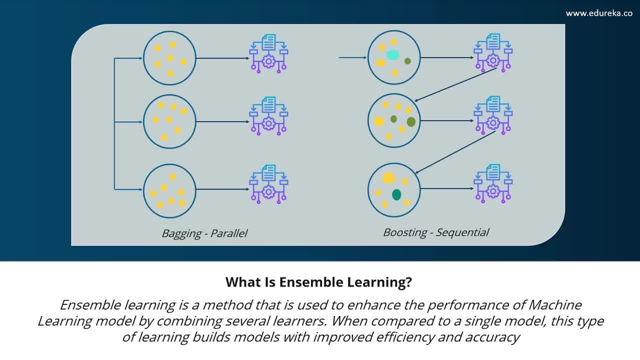 An example of bagging is the random forest algorithm. okay, So the principle behind bagging is you're dividing your data set into different bootstrap data sets and you're running a weak learner or an algorithm on each of these data sets, So you're parallelly doing all of this. 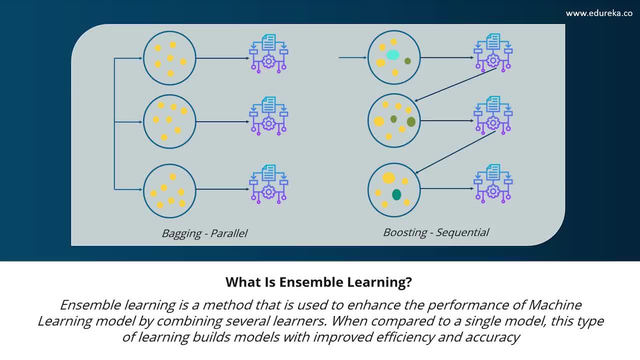 Whereas in boosting, you're sequentially doing this along with updating the weights depending on the misclassified samples, right? This is exactly what ensemble learning is, and I just told you what exactly bagging and boosting is Right, so there's a clear distinction between these two. 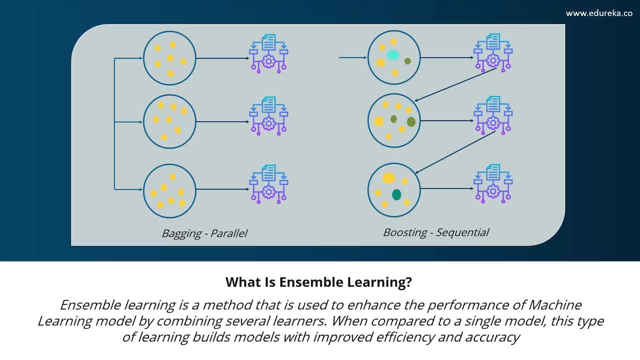 and this is actually one of the most frequently asked questions. If you go to an interview on machine learning, they always make sure to ask you what exactly is bagging and boosting, and how are they different? So let's make sure you understand the difference. 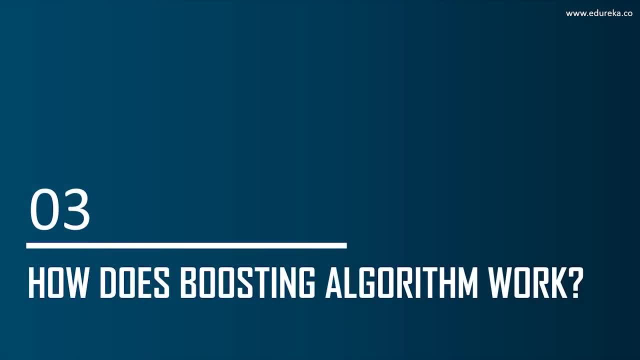 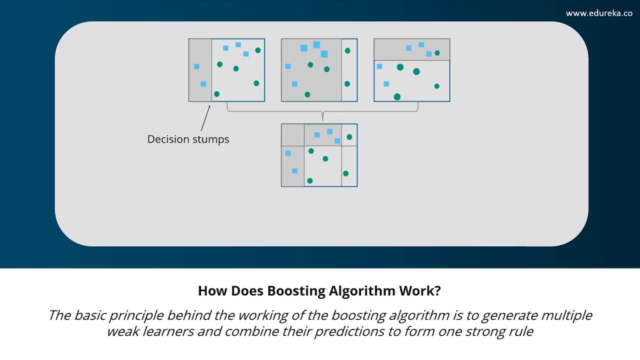 between the two. Now let's move on and understand how the boosting algorithm works. So, like I mentioned, the basic principle here is to generate multiple weak learners and combine their predictions to form one strong rule. Now these weak learners are generated by applying base machine learning algorithms. 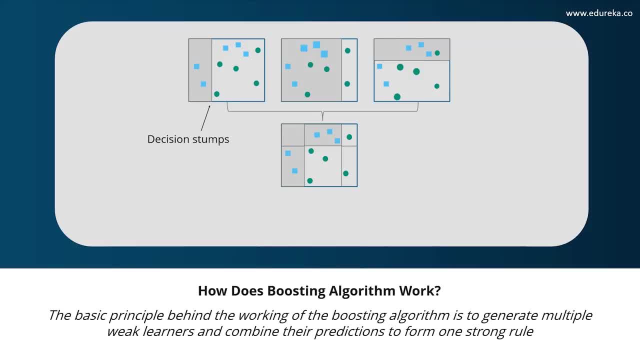 on different distributions of the data set. Now these base learning algorithms are usually decision trees by default in a boosting algorithm. So what these base learners do is they generate weak rules for each iteration. So after multiple iterations, the weak learners are combined and they form a strong learner. 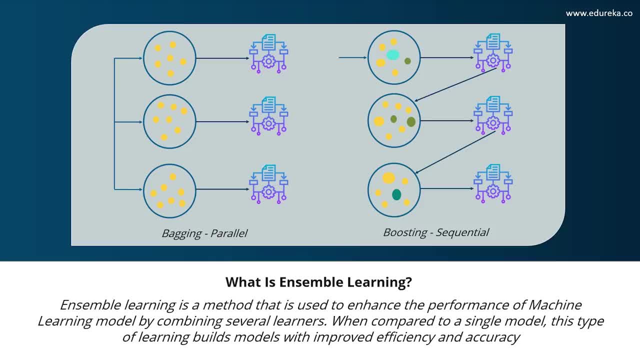 during the training phase. Now the performance of the model can be increased by parallelly training a number of weak learners on a bootstrap data set. an example of bagging is the random forest algorithm. Okay, So the principle behind bagging is: you're dividing your data set. 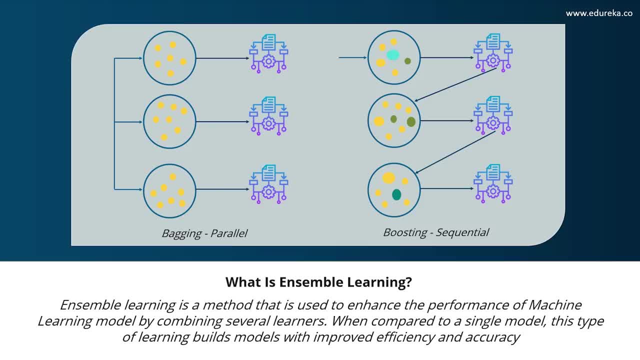 into different bootstrap data sets and you're running a weak learner or an algorithm on each of these data sets. So you're parallelly doing all of this, whereas in boosting your sequentially doing this, along with updating the weights depending on the misclassified samples, right? 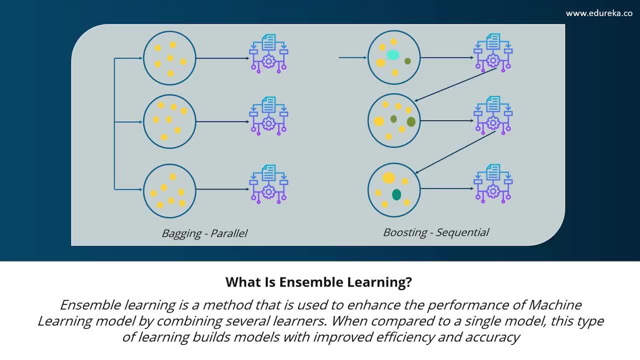 This is exactly what ensemble learning is, and I just told you what exactly bagging and boosting is right, So there's a clear distinction between these two, and this is actually one of the most frequently asked questions If you go for an interview on machine learning. 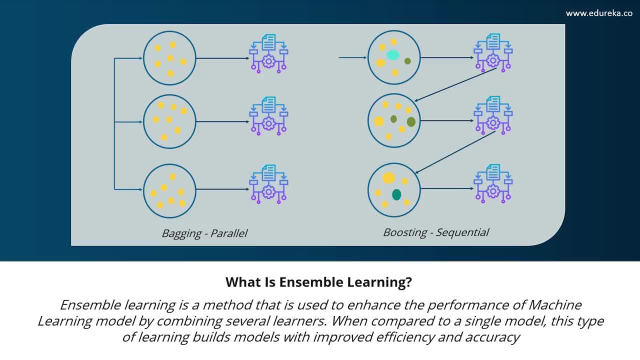 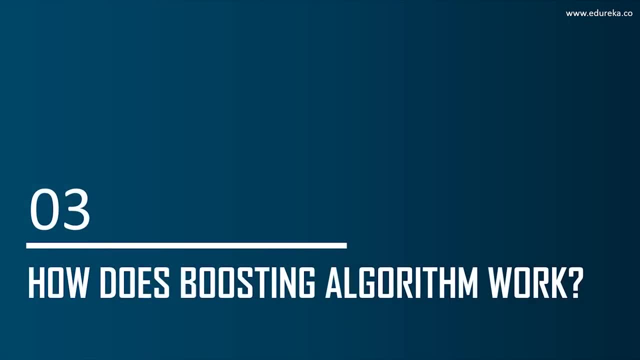 they always make sure to ask you what exactly is bagging and boosting and how are they different. So as make sure you understand the difference between the two. now let's move on and understand how the boosting algorithm works. So, like I mentioned, the basic principle here. 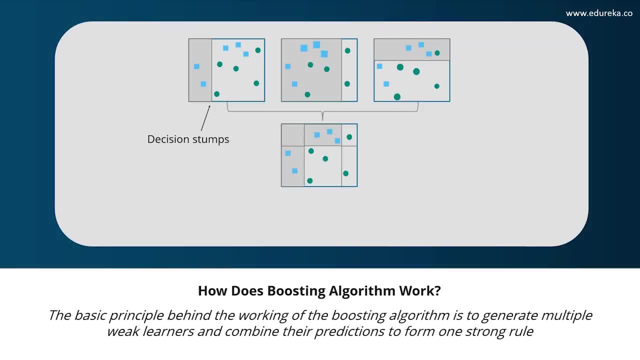 is to generate multiple weak learners and combine their predictions to form one strong rule. Now these weak learners are generated by applying base machine learning algorithms on different distribution of the data set. Now these base learning algorithms are usually decision trees by default in a boosting algorithm. 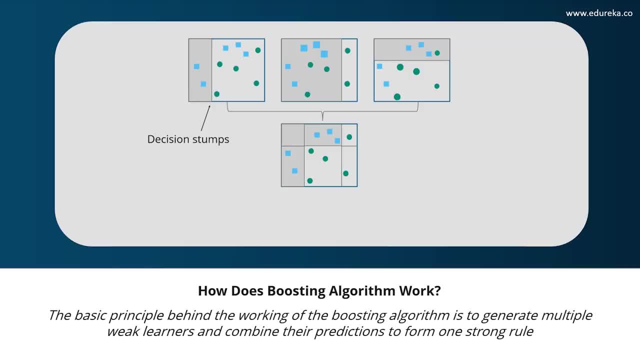 So what these base learners do is they generate weak rules for each iteration. So after multiple iterations, the weak learners are combined and they form a strong learner that will predict a more accurate outcome. So let me explain this stepwise to you. consider this about data set over here. 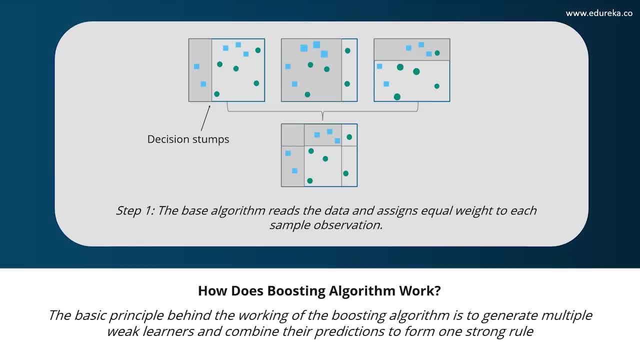 You have two different types of data. You have squares and you have circles, So, basically, your end goal is to classify them into two different classes. right, This is exactly how you do it. So how you start is: the base algorithm will read the data. 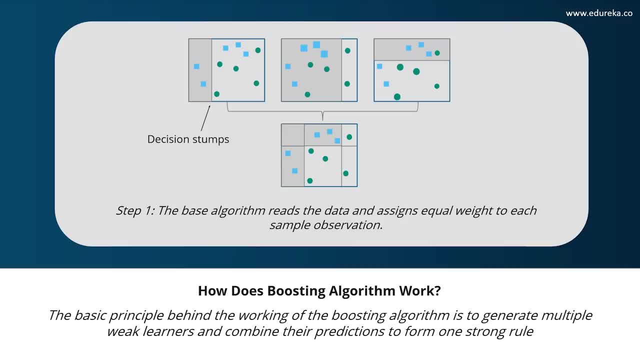 and it will assign equal weight to all of these data points. So after that I'll try to analyze the data and try to draw a decision stump. decision stump is basically a single level decision tree that tries to classify the data points. So after it assigns equal weightage to all the data points, 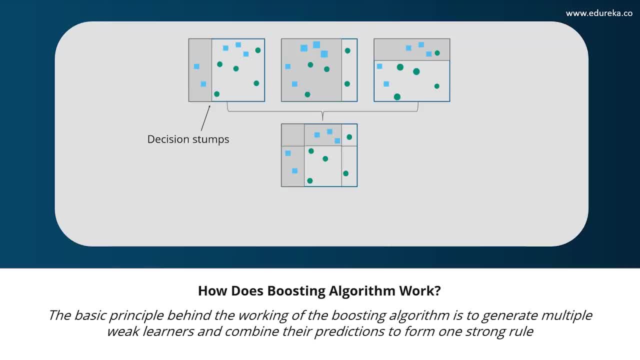 that will predict a more accurate outcome. So let me explain this stepwise to you. Consider this about data set over here You have two different types of data. You have squares and you have circles. So basically, your end goal is to classify them. 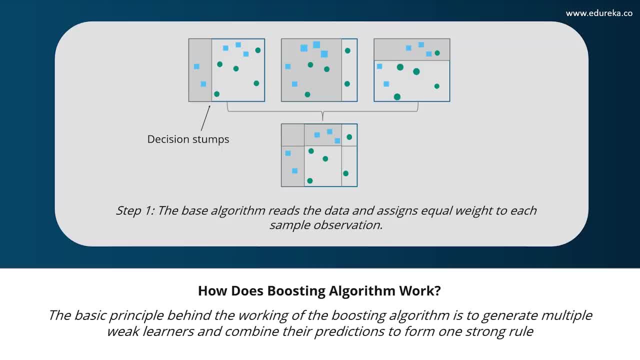 into two different classes. right, This is exactly how you do it. So how you start is: the base algorithm will read the data and it'll assign equal weight to all of these data points. So after that, I'll try to analyze the data. 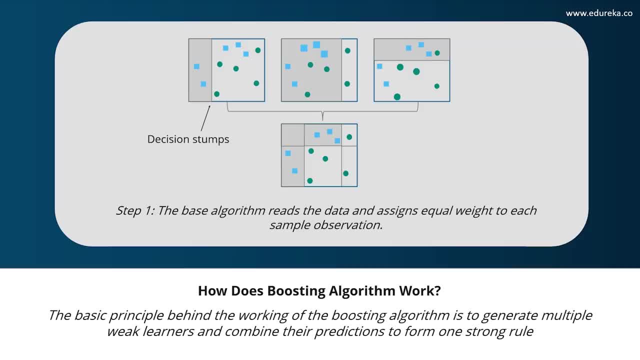 and try to draw a decision stump. Decision stump is basically a single level decision tree that tries to classify the data points. So after it assigns equal weightage to all the data points in the class, it will try to draw a decision stump right. 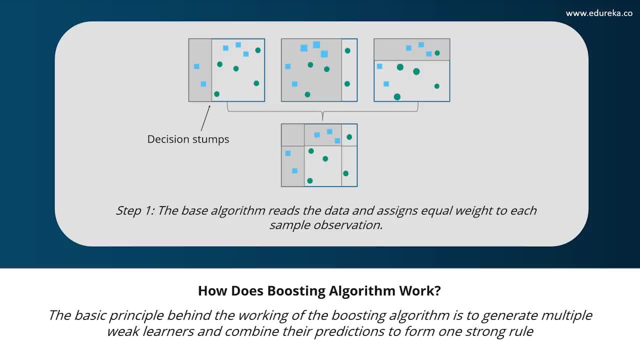 In the first image you can see the decision stump Now. after that, it'll check for any false predictions. Now the next step is the base learner will identify all the false predictions that it made. So in the next iteration, what you do is you just assign. 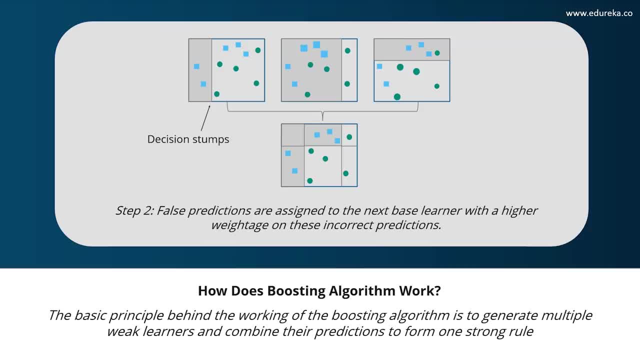 a higher weightage to these misclassified samples. In the first image, we've successfully separated these two squares right, But there are three other squares on the other side, meaning that we've misclassified these three squares. So in the next iteration- if you take a look at the image, 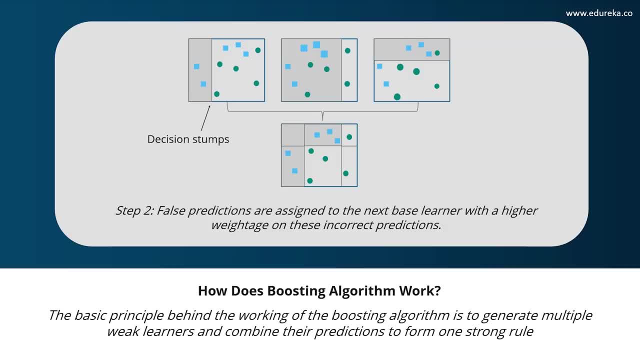 the three squares have a higher weightage, as in. I've shown that by increasing the size of the image. but yeah, the next iteration. you increase the weightage on your misclassified samples Similarly. you keep doing this until you separate your class A from your class B. 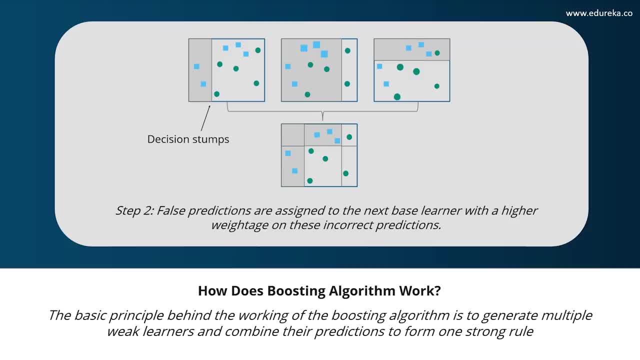 So, basically, you're going to pay more attention to your misclassified samples, You're going to increase their weightage and you're going to make sure that those samples are correctly Classified in the next iteration. So, like I said, you'll repeat the step two, right? 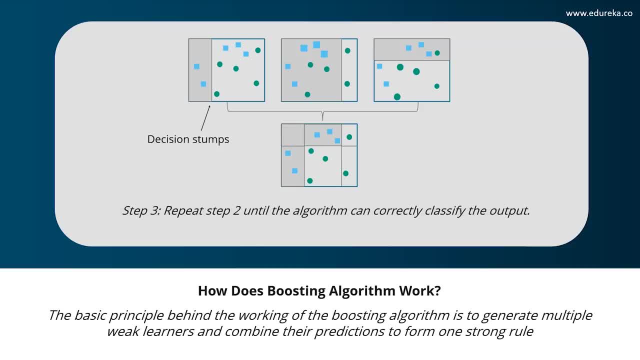 You will keep increasing the weightage of misclassified samples until all of the samples are correctly classified. So look at the fourth diagram here. So everything is classified correctly. right, We have a set of squares, We have a set of circles. So that's exactly how boosting algorithm works. 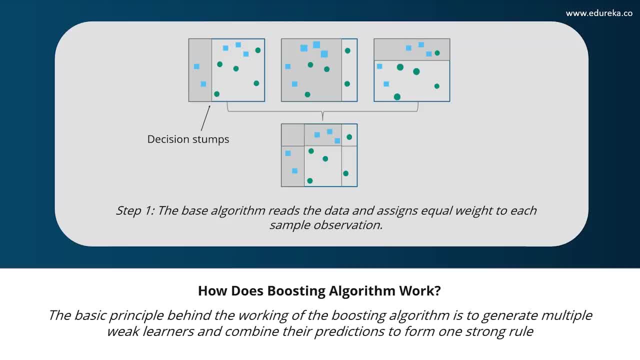 in the class It will try to draw a decision stump. right in the first image You can see the decision stump now. after that it will check for any false predictions. The next step is the base learner will identify all the false predictions that it made. 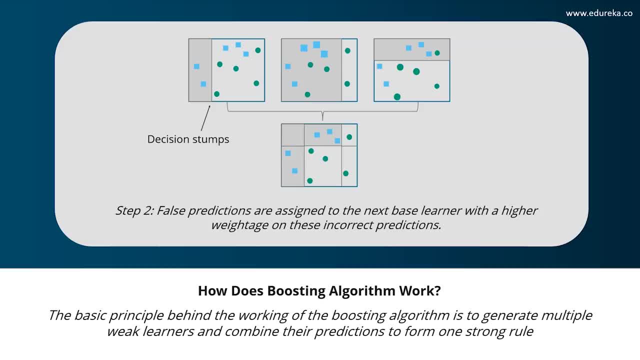 So in the next iteration, what you do is you just assign a higher weightage to these misclassified samples. in the first image, We have successfully separated these two squares, right, But there are three other squares on the other side, meaning that we've misclassified. 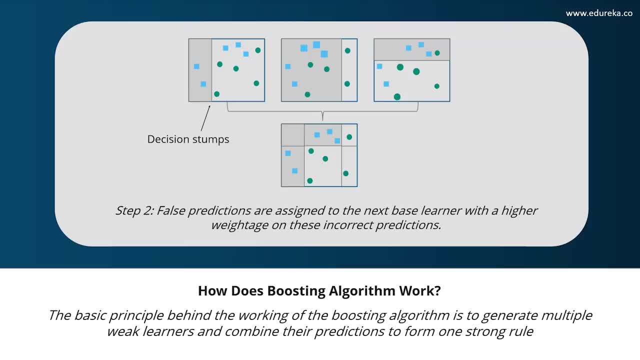 These three squares. So in the next iteration, if you take a look at the image, the three squares have a higher weightage, as in. I've shown that by increasing the size of the image. but yeah, the next iteration, you increase the weightage on your misclassified samples. 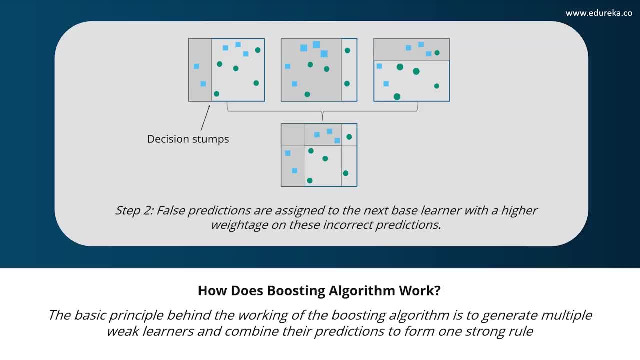 Similarly, you keep doing this until you separate your class a from your class B. So, basically, you're going to pay more attention to your misclassified samples, You're going to increase their weightage and you're going to make sure that those samples are correct. 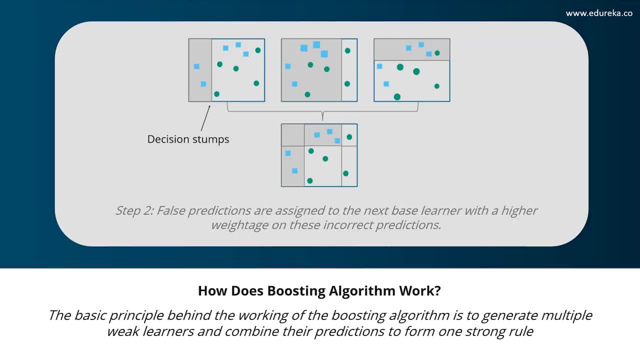 Lee classified in the next iteration. So, like I said, you'll repeat the step two, right? You will keep increasing the weightage of misclassified samples until all of the samples are correctly classified. So look at the fourth diagram here. So everything is classified correctly, right? 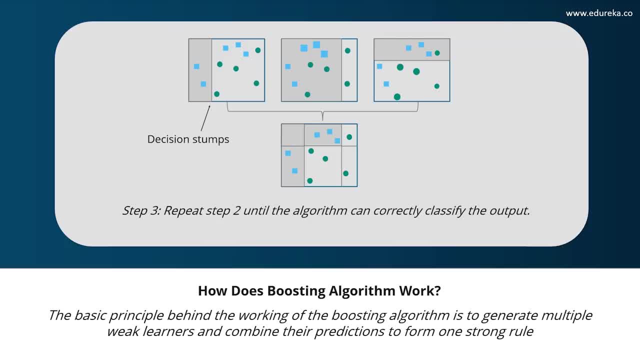 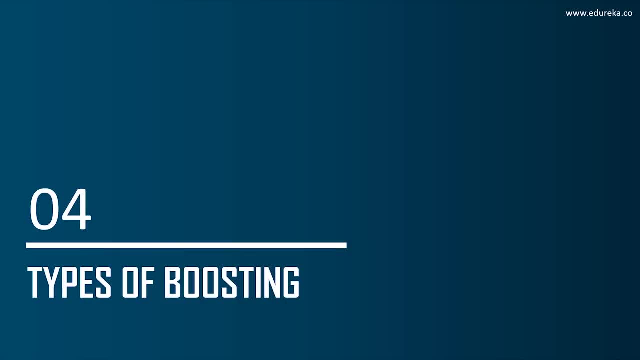 We have a set of squares, We have a set of circles, So that's exactly how boosting algorithm works. Now let's understand the different types of boosting. So mainly, there are three classes of boosting this: adaptive boosting, gradient boosting and XG boost. 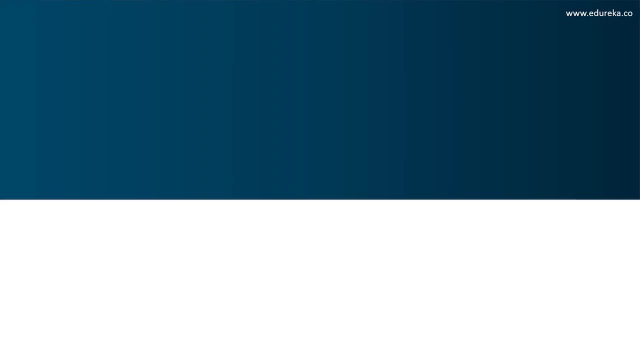 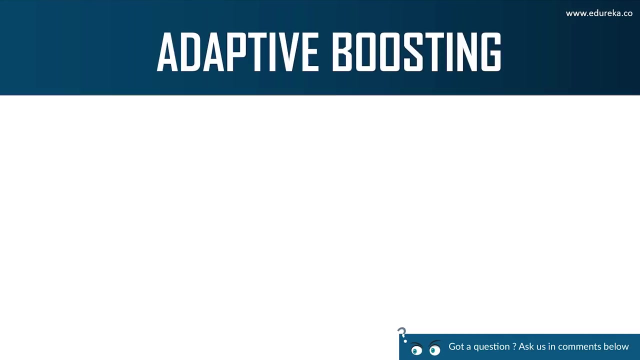 So we'll discuss each of these in brief. So adaptive boosting is what I explained to you in the previous slide. It is implemented by combining several weak learners into a single strong learner. So the couple of steps that this adaptive boosting algorithm follows. so adaptive boosting starts by assigning equal weightage. 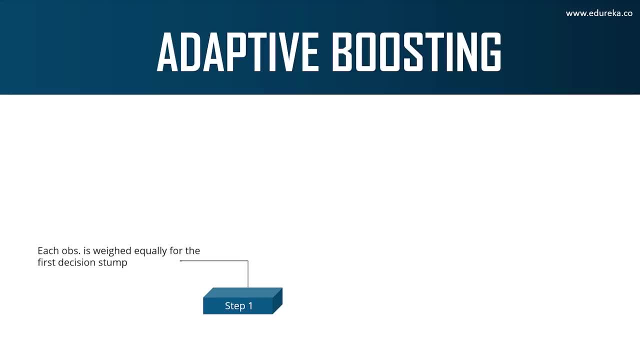 to all of your data points and you draw out a decision stump for a single input feature. So the next step is the results that you get from the first decision stump are analyzed and if any observations are misclassified, then they are assigned higher weights. 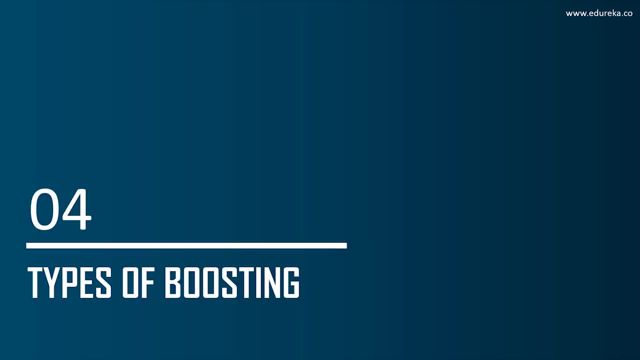 Now let's understand the different types of boosting. So mainly, there are three classes of boosting: this: adaptive boosting, gradient boosting and XG boost. So we'll discuss each of these in brief. So adaptive boosting is what I explained to you in the previous slide. 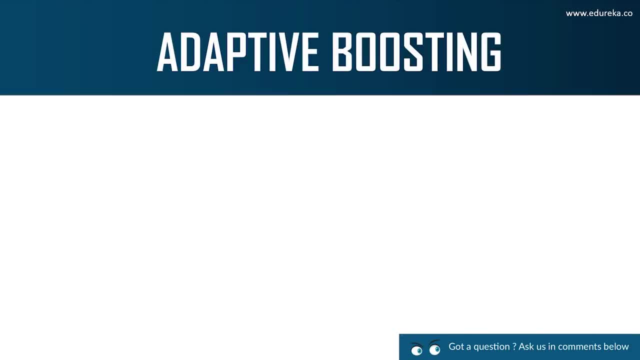 It is implemented by combining several weak learners into a single strong learner. So there are a couple of steps that this adaptive boosting algorithm follows. So adaptive boosting starts by assigning equal weightage to all of your data points and you draw out a decision stump for a single input feature. 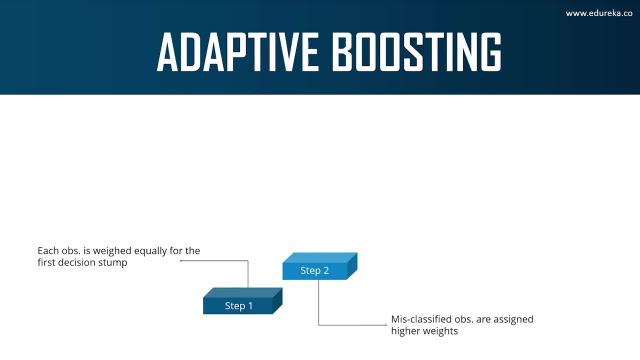 So the next step is the results that you get from the first decision Decision stump are analyzed and if any observations are misclassified, then they are assigned higher weights. This is exactly what I explained in the previous slide also. So after that, new decision stump is drawn. 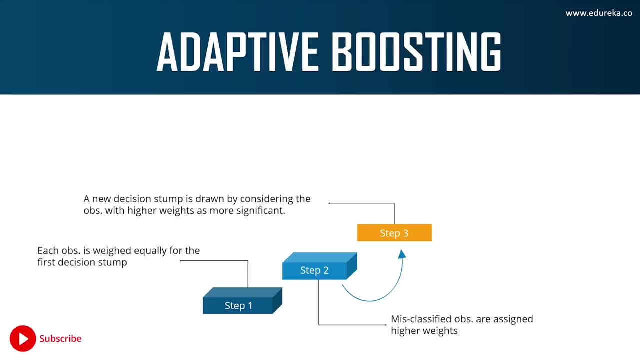 by considering the observations with the higher weights as more significant, So whichever data point was misclassified, they are given a higher weightage. In the next step, you'll draw another decision stump that tries to classify the data points by giving more importance to the data points with higher weightage. 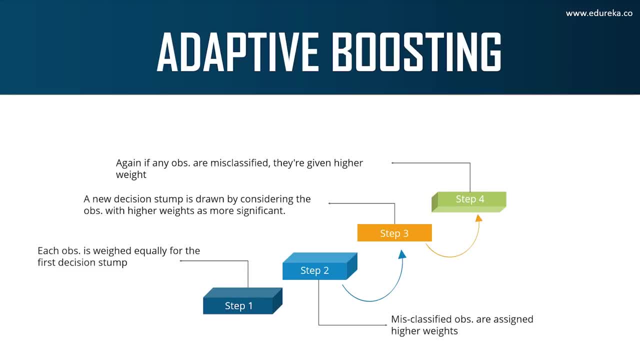 Again, if there are any observations that are misclassified, then they're given higher weight, and this process will keep continuing. It'll keep looping until all the observations fall into the right class. So the end goal here is to make sure that all your data points are classified. 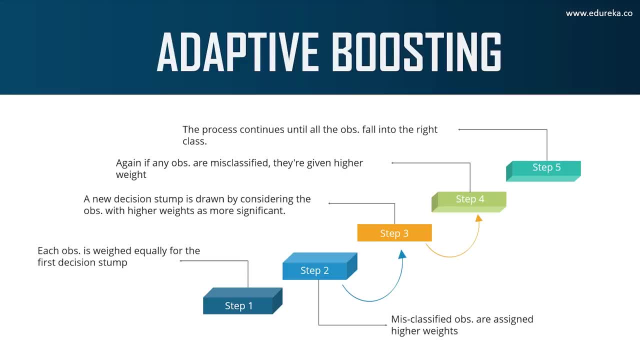 into the correct classes. Adaptive boosting, or add a boost, can also be used for regression problems. It's not restricted to classification only. It can be used for both classification and regression, But it's more commonly seen in classification problems. So that was a brief about adaptive boosting. 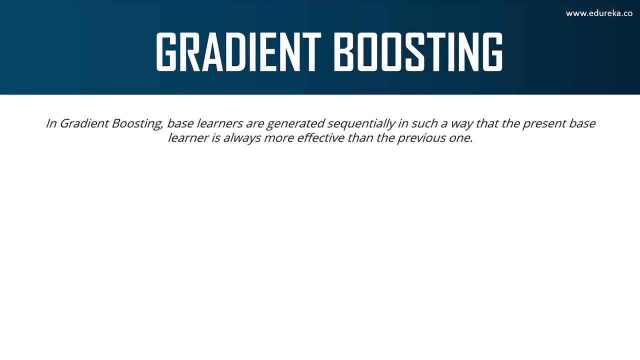 Now let's understand gradient boosting. So gradient boosting is also based on the sequential ensemble learning model. Here what happens is the base learners are generated sequentially in such a way that the present base learner is always more effective than the previous one. Basically, the overall model improves sequentially. 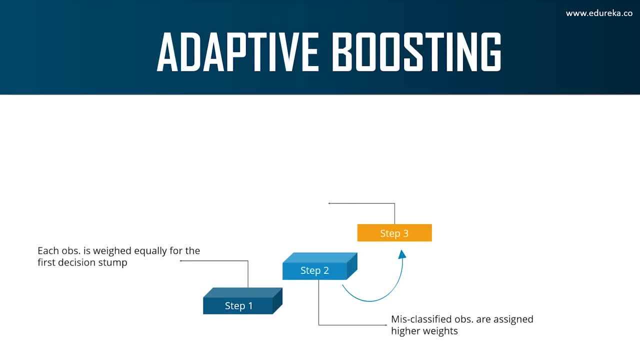 This is exactly what I explained in the previous slide also. So after that, new decision stump is drawn by considering the observations with the higher weights as more significant. So whichever data point was misclassified, they are given a higher weightage in the next step. 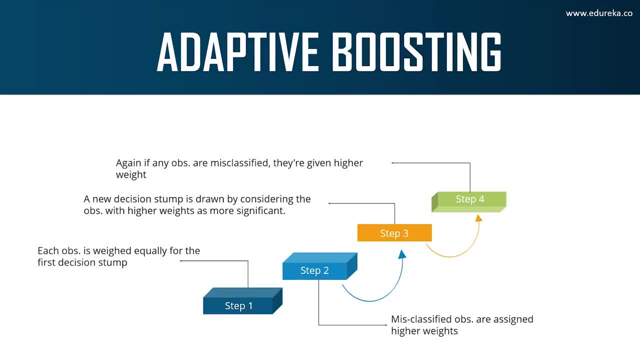 You'll draw another decision stump that tries to classify the data points by giving more importance to the data points with higher weightage. again, if there are any observations that are misclassified, then they're given higher weight and this process will keep continuing and keep looping until all the observations fall. 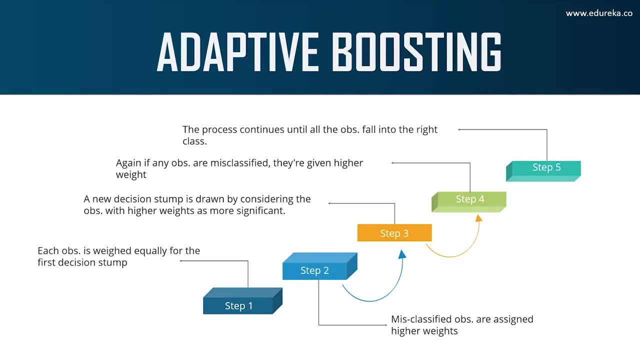 into the right class. So the end goal here is to make sure that all your data points are classified into the correct classes. adaptive boosting- or add a boost- can also be used for regression problems. It's not restricted to classification only. it can be used for both. 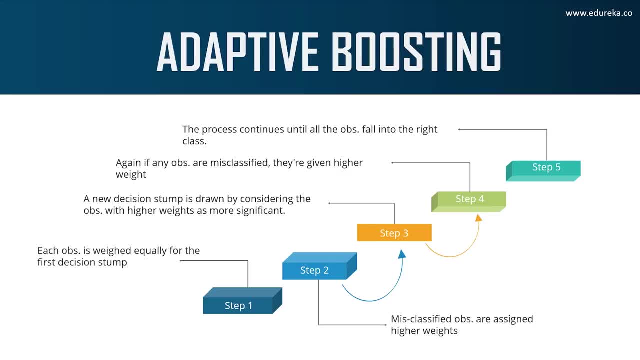 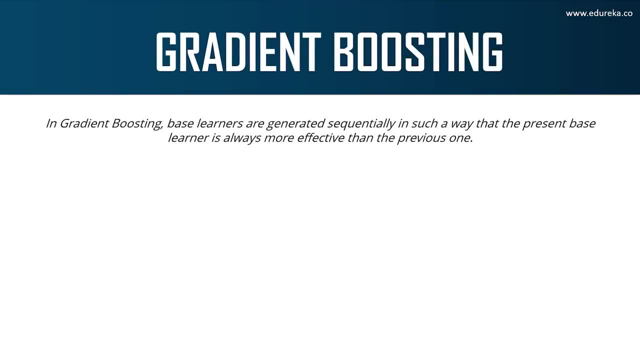 It can be used for classification and regression, but it's more commonly seen in classification problems. So that was a brief about adaptive boosting. Now let's understand gradient boosting. So gradient boosting is also based on the sequential ensemble learning model. here What happens is the base learners are generated sequentially. 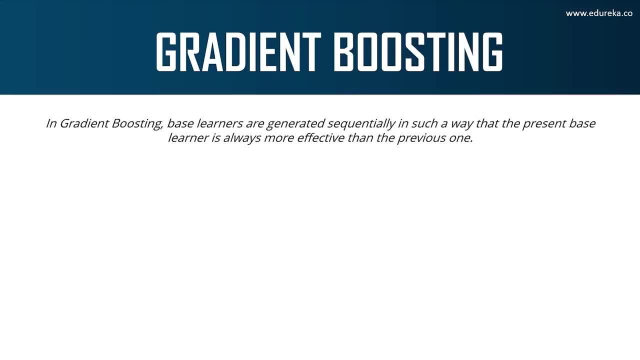 in such a way that the present based learner is always more effective than the previous one. Basically, the overall model improves sequentially with each iteration. Now, the difference in this type of boosting is that the weights for misclassified outcomes are not incremented. You're not going to increment or add weights. 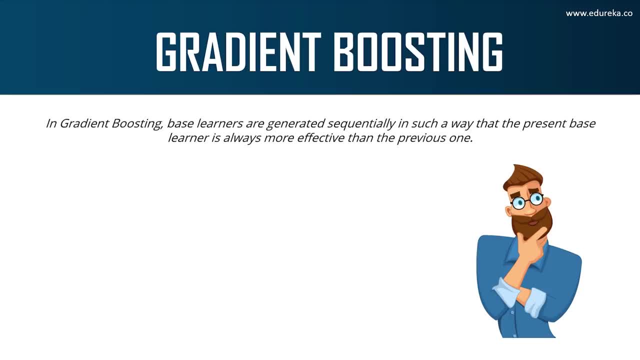 to the misclassified outcomes instead in gradient boosting, What you do is you try to optimize the loss function of the previous learner by adding a new adaptive model that adds weak learners in order to reduce the loss function. Now, the main idea here is to overcome the errors. 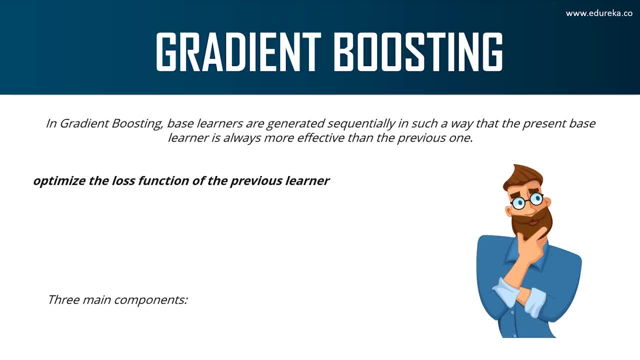 in the previous learners prediction. Now, this type of boosting has three main components. It has something known as the loss function. Loss function is the one that needs to be optimized, meaning that you need to reduce the error. The other component is that the weak learners are needed. 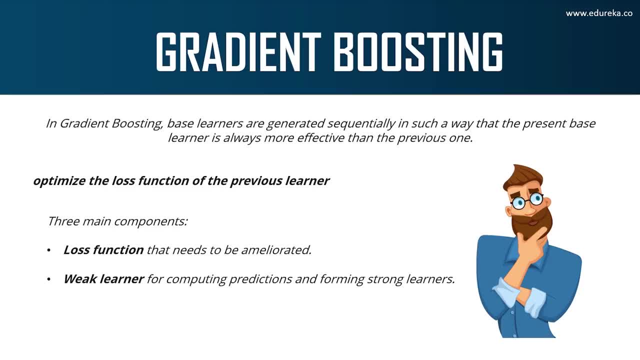 for computing predictions and forming strong learners, Then you'll need an additional model that will regularize the loss function, meaning that it will try to fix the loss or the error from the previous weak learner Right. so you keep adding a model that will regularize the loss function. 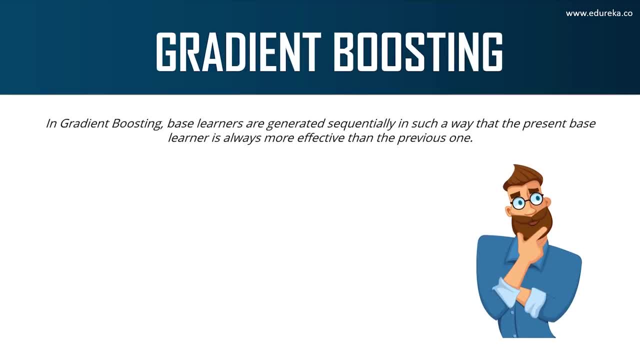 with each iteration. Now, the difference in this type of boosting is that the weights for misclassified outcomes are not incremented. You're not going to increment or add weights to the misclassified outcomes. Instead, in gradient boosting, what you do is you try to optimize the loss function. 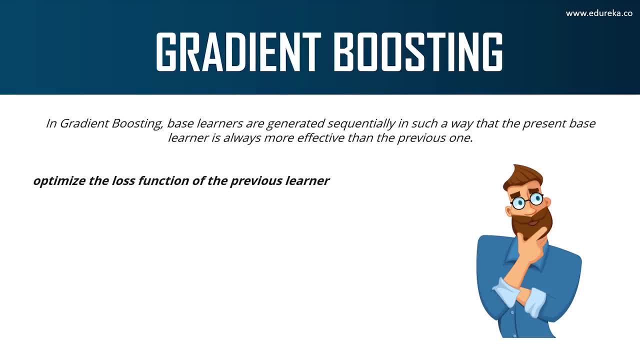 of the previous learner by adding a new adaptive model that adds weak learners in order to reduce the loss function. Now, the main idea here is to overcome the errors in the previous learner's prediction. Now, this type of boosting has three main components. It has something known as the loss function. 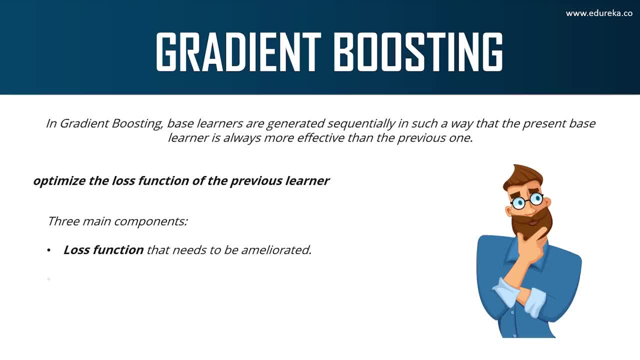 Loss function is the one that needs to be optimized, meaning that you need to reduce the error. The other component is that the weak learners are needed for computing predictions and forming strong learners. Then you'll need an additional model that will regularize the loss function. 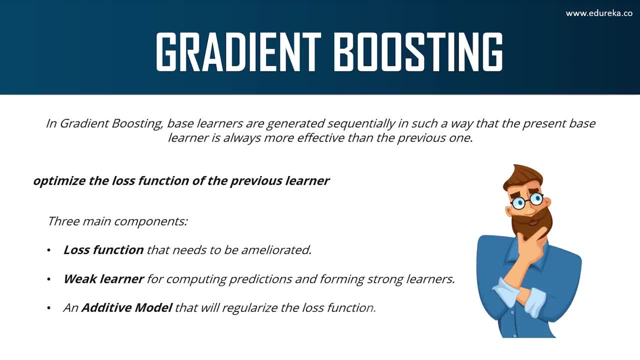 meaning that it will try to fix the loss or the error from the previous weak learner Right. so you keep adding a model that will regularize the loss function from the previous learner. So, just like adaptive boosting, gradient boosting can also be used for both classification and regression problems. 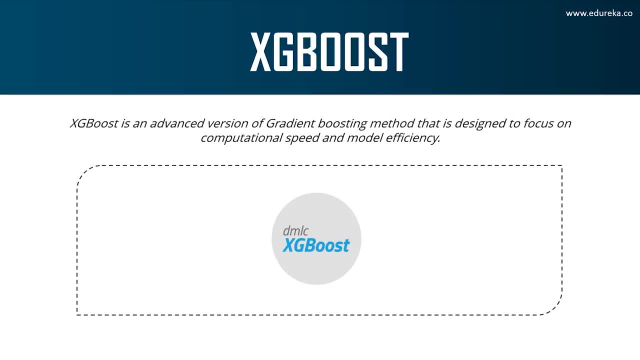 Now let's discuss the last type of boosting, which is XGBoost. Now, XGBoost is basically an advanced version of gradient boosting. It literally means extreme gradient boosting. So XGBoosting actually falls under the category of distributed machine learning community. 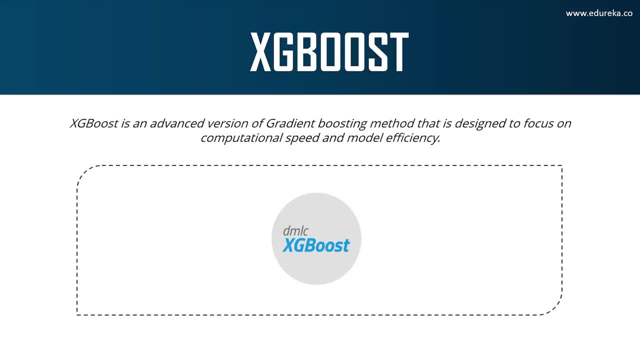 Okay, it's a more advanced version of the gradient boosting method. The main aim in this algorithm is to increase the speed and to increase the efficiency of your computations and of the model performance. So the reason why this model was introduced was because gradient boosting algorithm was computing the output. 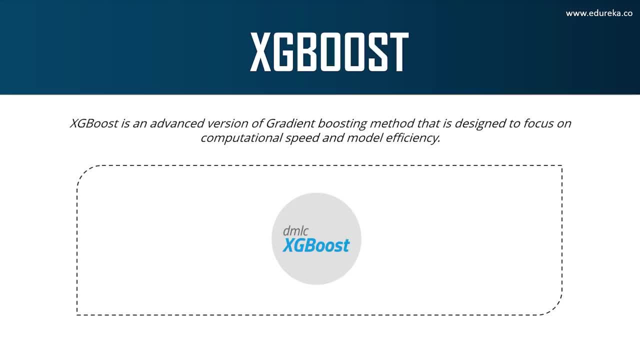 at a very slow rate. right, Because there's sequential analysis of the data set and it takes a longer time. That's why XGBoost was introduced. It basically boosts, or extremely boosts, the performance of the model. So XGBoost is mainly going to focus on your speed. 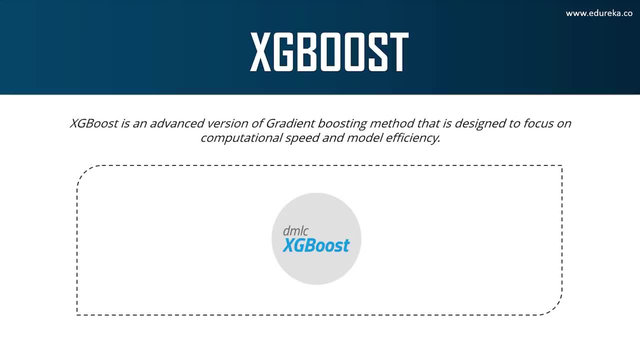 and your model efficiency. In order to do this, it has a couple of features. It supports parallelization by creating decision trees parallelly. There's no sequential modeling in this. It implements something known as distributed computing methods for evaluating any large and any complex models. 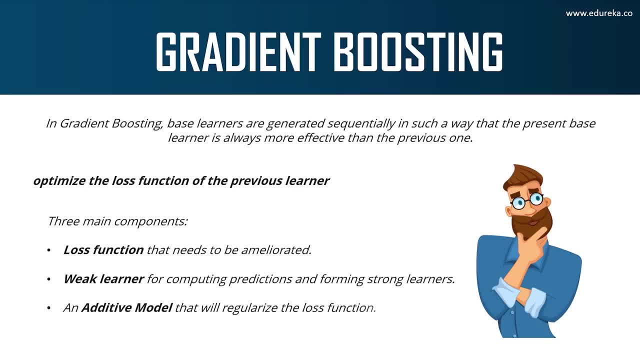 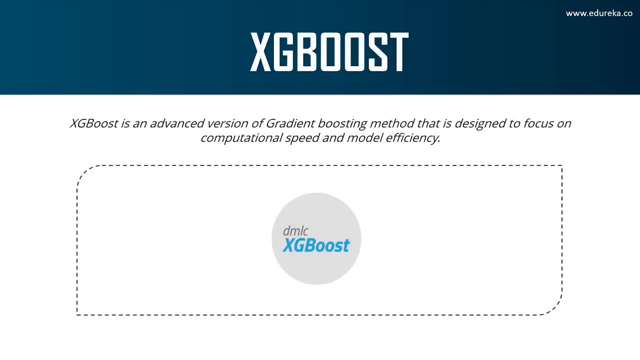 from the previous learner. So, just like adaptive boosting, gradient boosting can also be used for both classification and regression problems. Now let's discuss the last type of boosting, which is XG boost. Now, XG boost is basically an advanced version of gradient boosting. 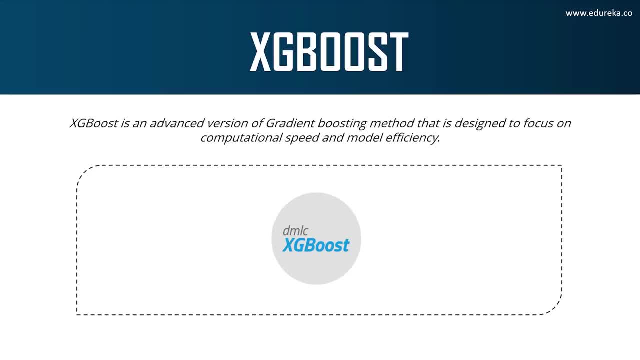 It literally means extreme gradient boosting. So XG boosting actually falls under the category of distributed machine learning Community. Okay, it's a more advanced version of the gradient boosting method. The main aim in this algorithm is to increase the speed and to increase the efficiency of your computations. 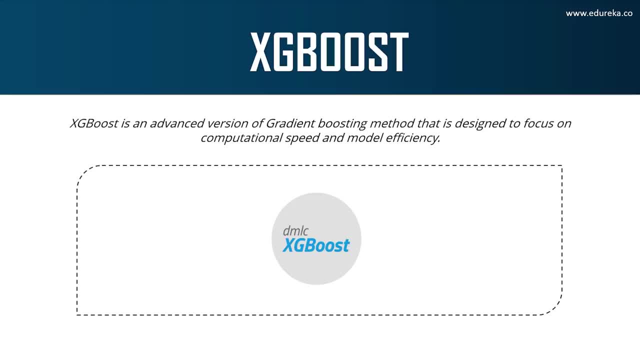 and of the model performance. So the reason why this model was introduced was because gradient boosting algorithm was computing the output at a very slow rate. right, because there's sequential analysis of the data set and it takes a longer time. That's why XG boost was introduced. 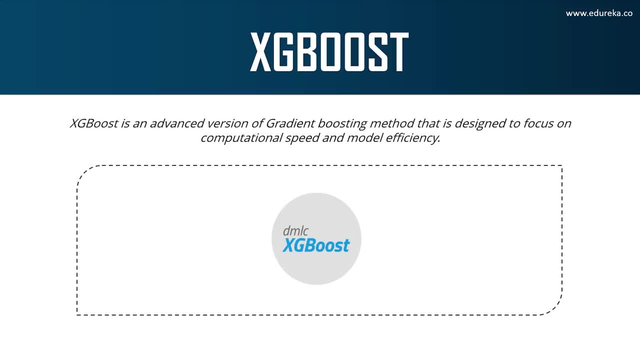 It basically boosts your, or extremely boost the performance of the model. So XG boost is mainly going to focus on your speed and your model efficiency. in order to do this, It has a couple of features. It supports parallelization by creating decision trees parallelly. 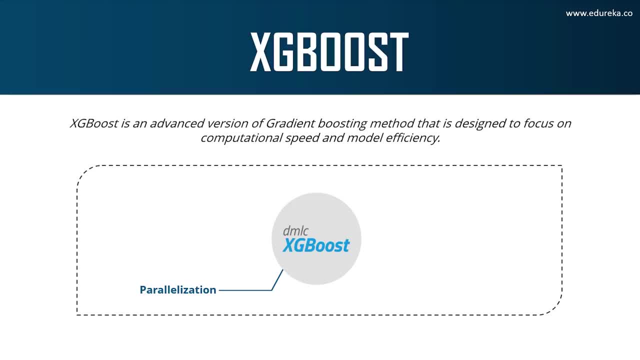 There's no sequential modeling in this. it implements something known as distributed computing methods for evaluating any large and any complex models. It also uses out-of-court computing in order to analyze huge and varied data sets. it implements cache optimization in order to make best use of your hardware. 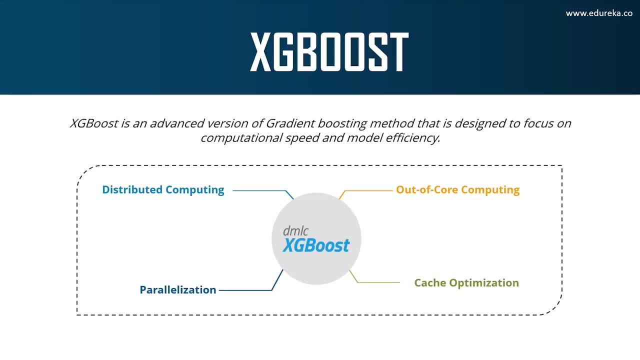 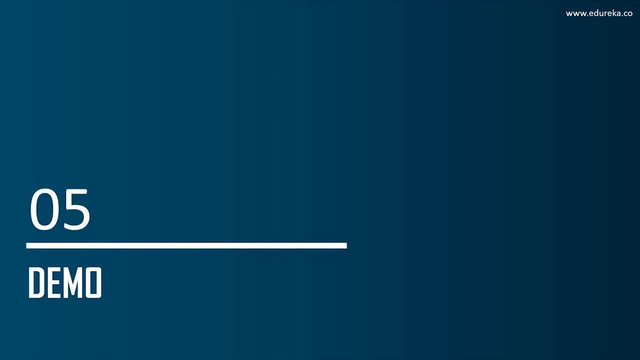 and of your resources overall. So, guys, these were the basics of the different types of boosting algorithms. now, to make things a little more interesting, Let's run a practical implementation. a short disclaimer before I get started with the demo is that I'll be using Python. 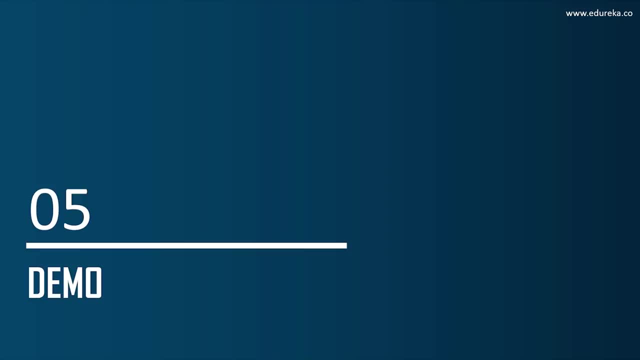 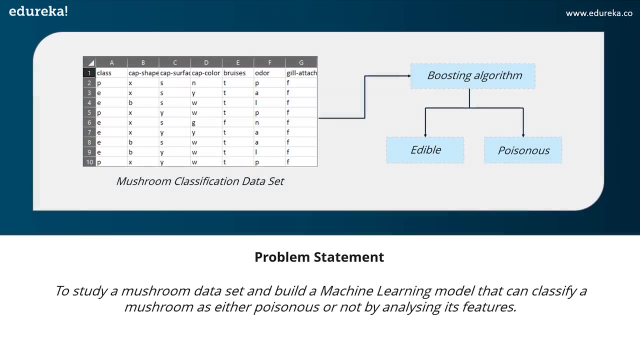 to run this demo. So if you don't know Python, I'll leave a couple of links in the description box. You can go through those links and maybe then come back and watch this video. So now let's understand what exactly we're going to do. 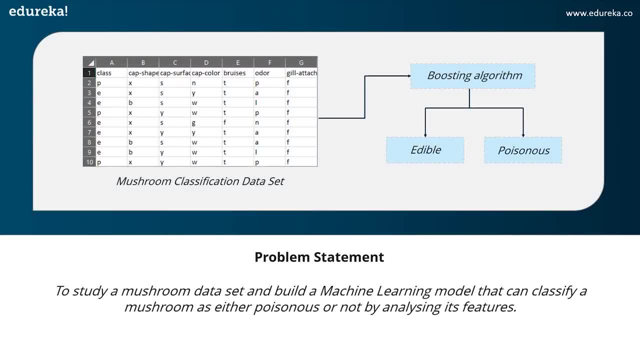 in this demo. So your problem statement is to study a mushroom data set and build a machine learning model that can classify a mushroom as either poisonous or edible by analyzing the features of the mushroom. So you're going to be given a mushroom data set. 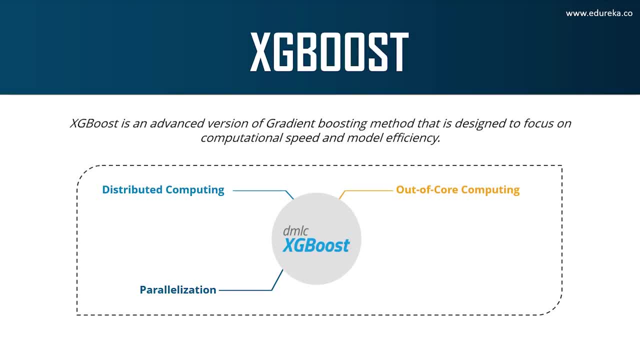 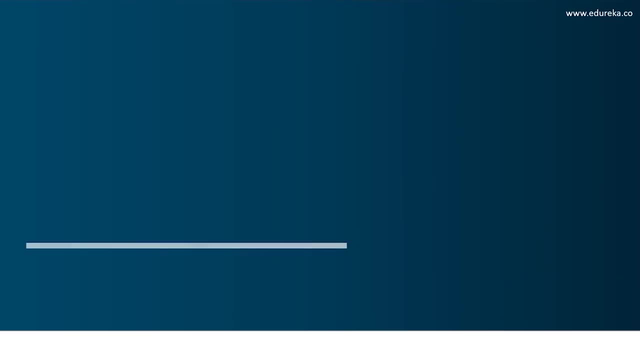 It also uses out-of-court computing in order to analyze huge and varied data sets. It implements cache optimization in order to make best use of your hardware and of your resources overall. So, guys, these were the basics of the different types of boosting algorithms. 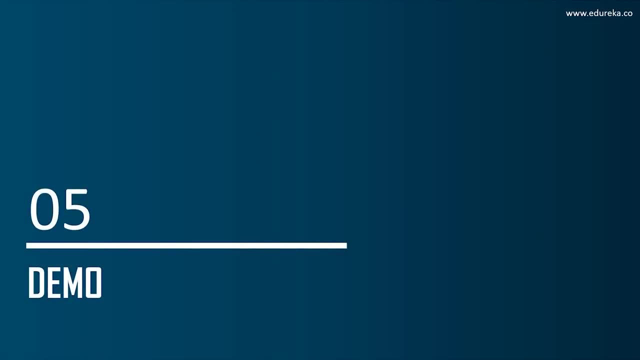 Now, to make things a little more interesting, let's run a practical implementation. A short disclaimer before I get started with the demo is that I'll be using Python to run this demo, So if you don't know Python, I'll leave a couple of links in the description. 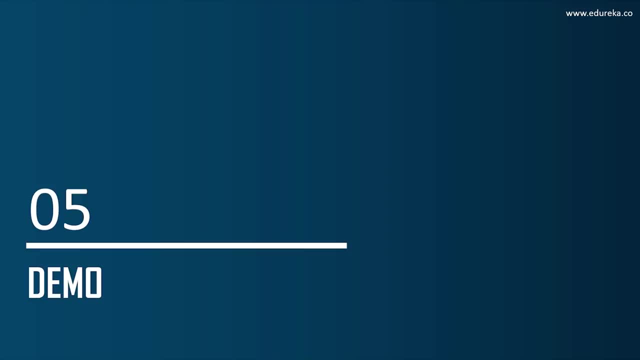 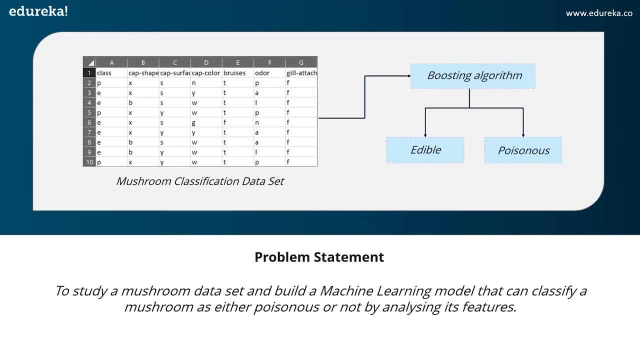 box. you can go through those links and maybe then come back and watch this video. So now let's understand what exactly we're going to do in this demo. So your problem statement is to study a mushroom data set and build a machine learning model. 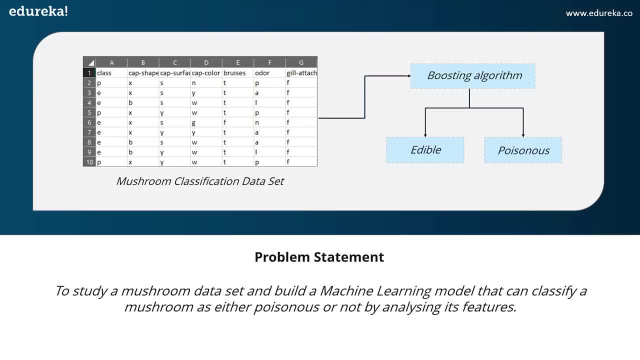 that can classify a mushroom as either poisonous or edible by analyzing the features of the mushroom. So you're going to be given a mushroom data set. What you have to do is you have to understand which of these mushrooms are edible and which is poisonous. 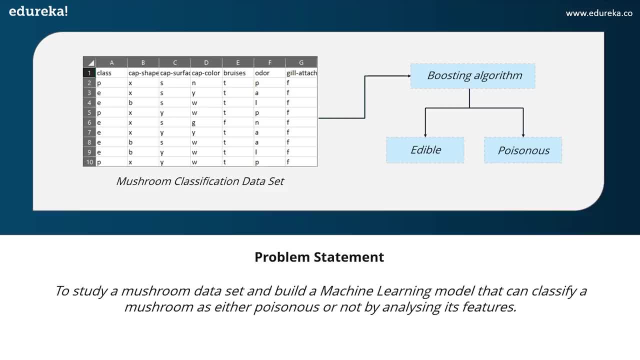 So this data set basically has mushrooms of 23 different species, and each species is either classified as edible mushrooms or non-edible ones, right? So, guys? the logic again over here is to build a machine learning model by using one of the boosting algorithms in order to predict whether 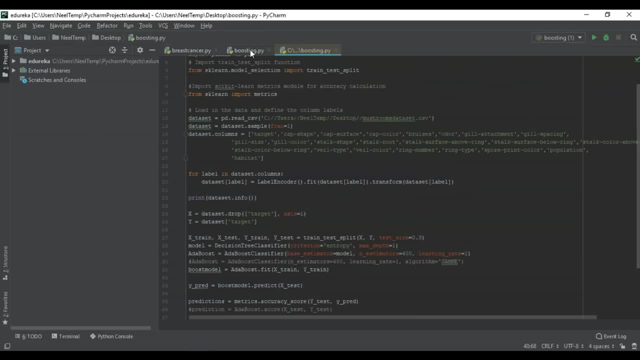 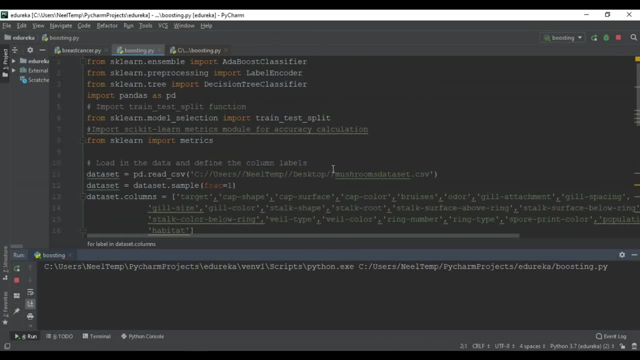 or not a mushroom is edible, So let me quickly open up the code for you. I hope all of y'all can see the console, So we'll wait for this to run. Until then, let me just run you through the entire code. 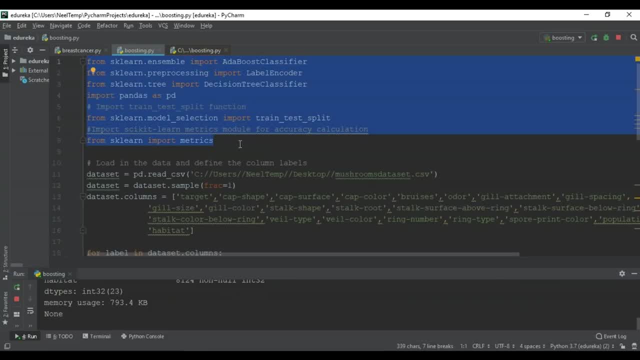 So, like any other demo, what you do is you start by importing the required packages. Now, the best thing in Python is that there are inbuilt packages and libraries which will let you implement any complex process. All you have to do is you have to import these libraries. 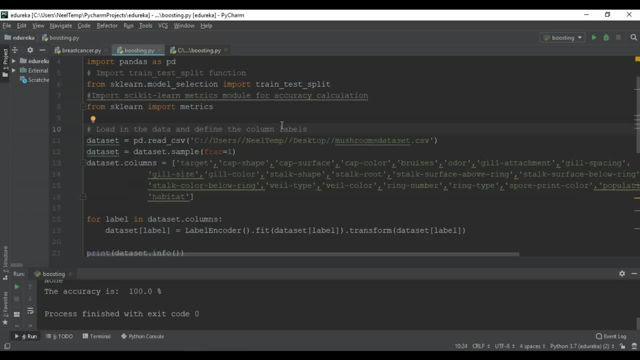 So that's exactly what I'm doing over here. After that, I'm loading the data set into a variable known as data set. So, basically, this is my data set. It's stored in this location. All I'm doing is I'm reading it. 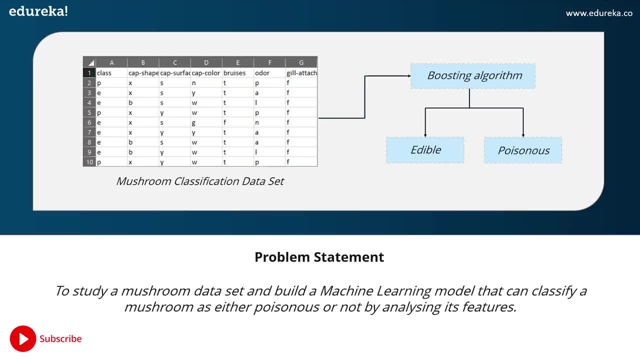 What you have to do is you have to understand Which of these mushrooms are edible and which is poisonous. So this data set basically has mushrooms of 23 different species, and each species is either classified as edible mushrooms or non-edible ones, right? 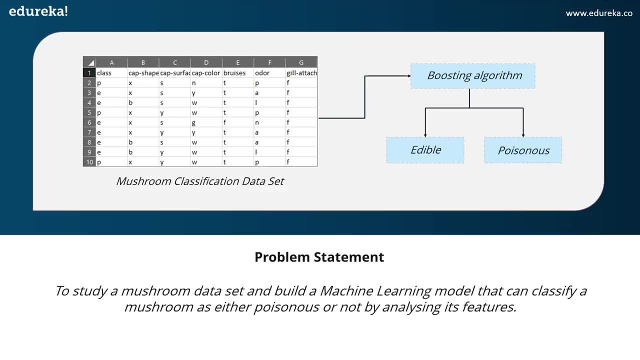 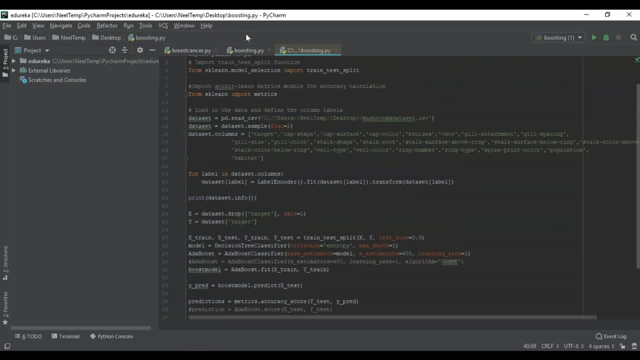 So, guys, the logic again over here is to build a machine learning model by using one of the boosting algorithms in order to predict whether or not a mushroom is edible. So let me quickly open up the code for you. I hope all of y'all can see the console. 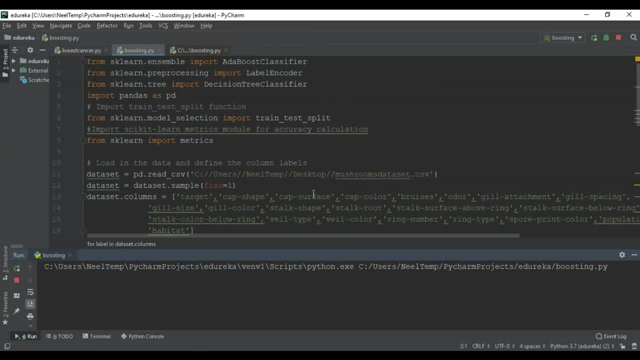 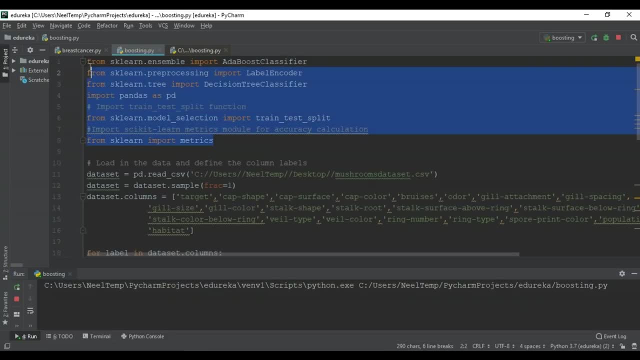 So we'll wait for this to run. until then, Let me just run you through the entire code. So, like any other demo, what you do is you start by importing the required packages. Now, the best thing in python is that there are inbuilt packages and libraries. 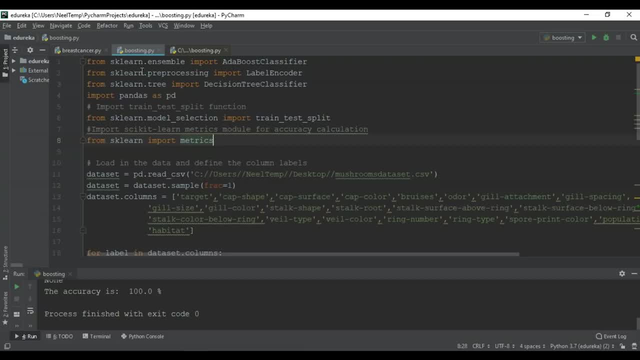 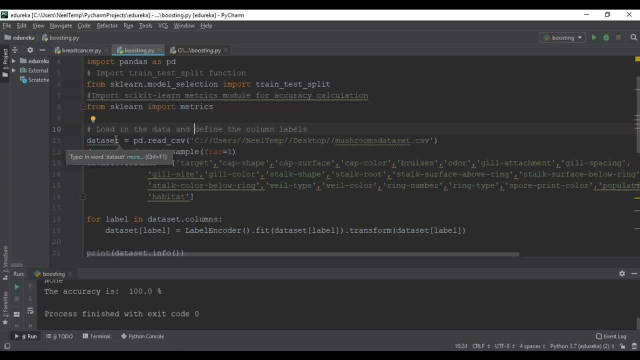 which will let you implement any complex process. All you have to do is you have to import these libraries. So that's exactly what I'm doing over here. after that, I'm loading the data set into a variable known as data set. That's basically. this is my data set. 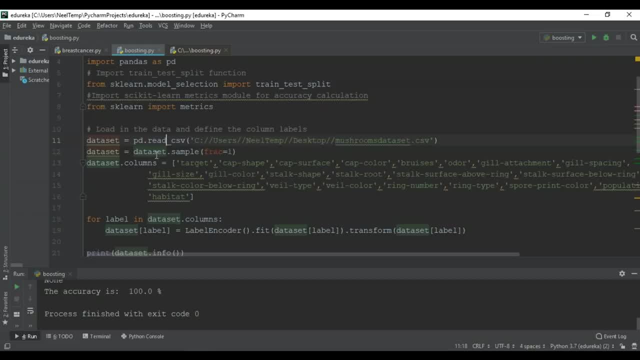 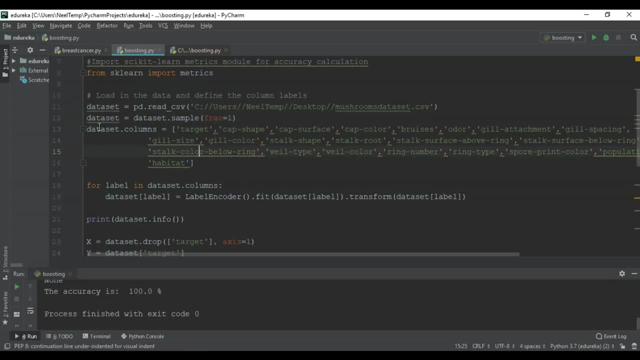 It's stored in this location at. all I'm doing is I'm reading it and I'm storing it in this variable. after that we'll perform data processing here. We'll define the column names right in our data set. The column names are not defined. 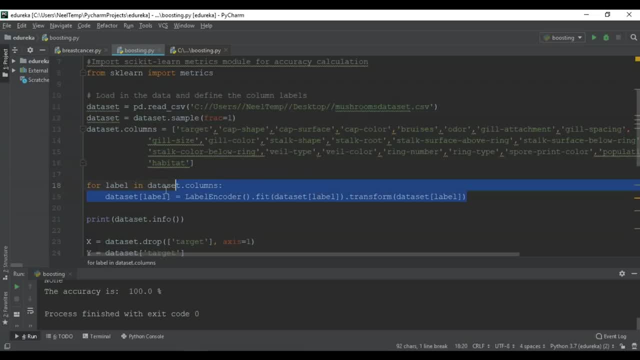 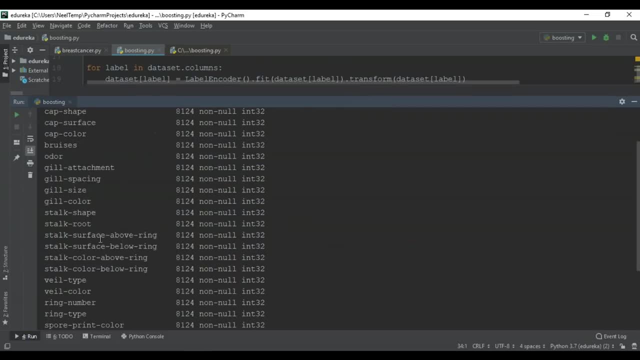 and I'm just defining all the column names here and then we're assigning these column names to our data set. next We're running this print data set, dot info, to look at all our features. So these are our data columns. So in total we have 23 features meaning. 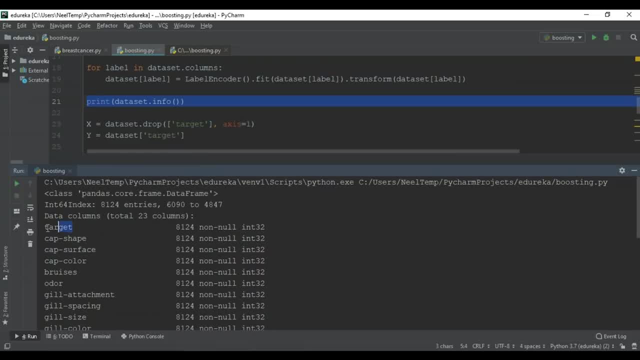 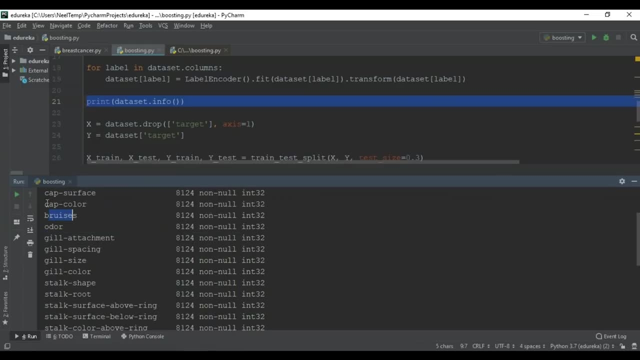 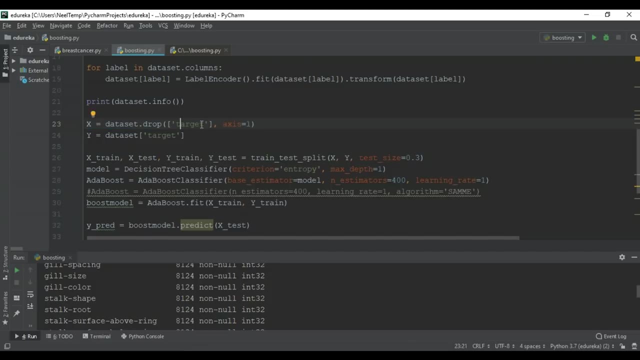 that there are 23 variables are, to which one variable is your target variable. So the target variable is your output variable that we're trying to predict, and the rest of the variables- bruises, cap, color, cap, surface- All of these are predictor variables. next, What we're going to do is we're going to drop this target variable. 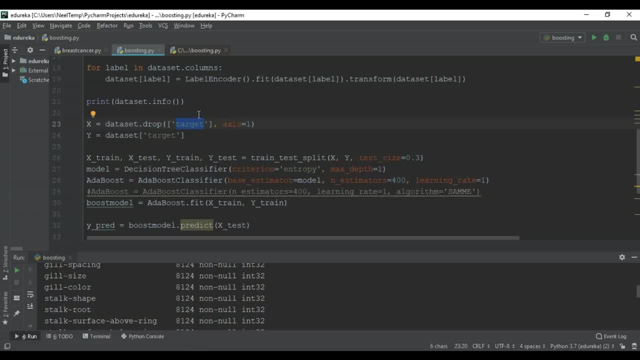 from our data set because we're trying to predict this. we're trying to predict the value of this target variable, So we'll just drop this variable because we are trying to predict that variable, or why will contain our target variable, or X will contain no target variable. now 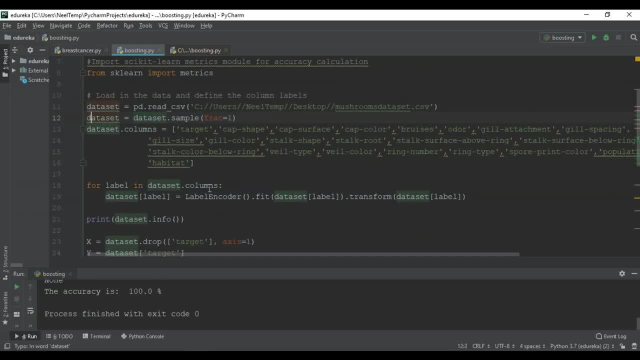 and I'm storing it in this variable. After that we'll perform data processing here. We'll define the column names In our data set. the column names are not defined and I'm just defining all the column names here And then we're assigning these column names to our data set. 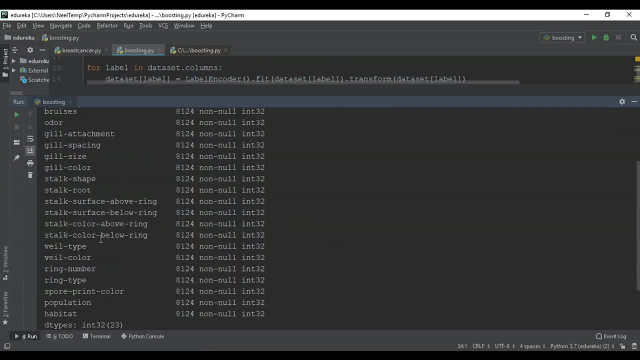 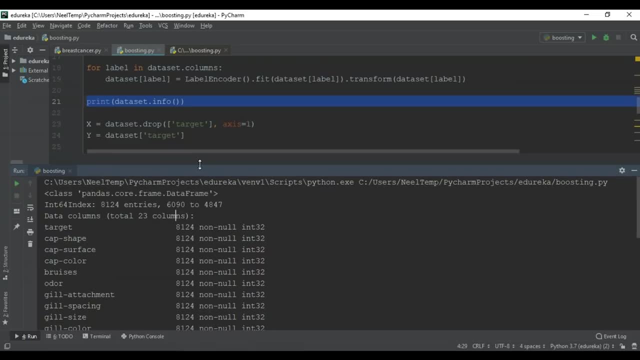 Next we're running this print data setinfo to look at all our features. So these are our data columns. So in total we have 23 features, meaning that there are 23 variables, out of which one variable is your target variable. 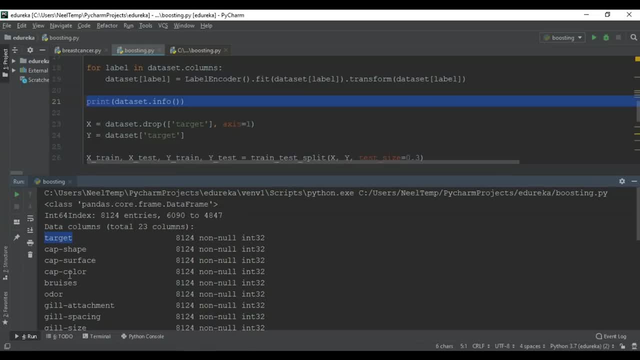 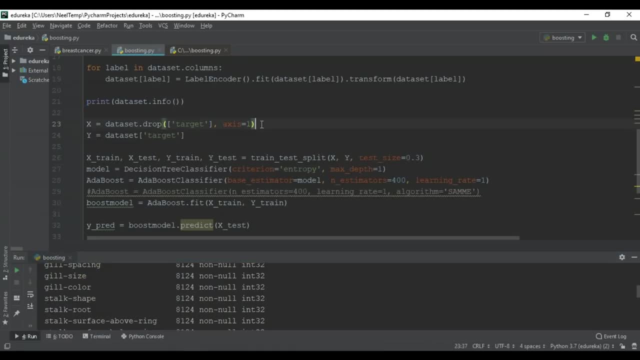 So the target variable is your output variable that we're trying to predict, and the rest of the variables- bruises, cap, color, cap, surface- all of these are predictor variables. Next, what we're going to do is we're going to drop this target variable from our data set. 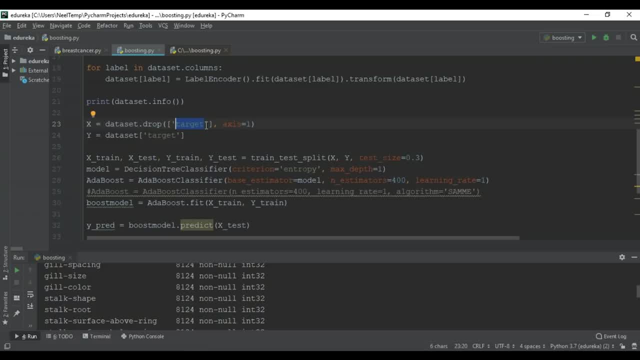 because we're trying to predict this. We're trying to predict the value of this target variable, So we'll just drop this variable because we are trying to predict that variable. Our Y will contain our target variable. Our X will contain no target variable. 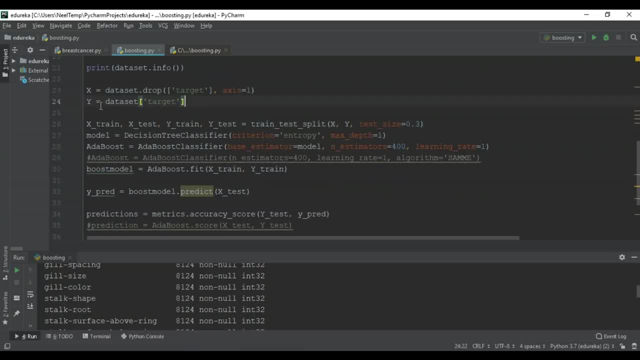 Now Y is basically created for evaluating your model. So, guys, I hope you all know what all of this is right. I'm not going in-depth into this because this is basic machine learning, and I'm hoping that you all have a good idea. 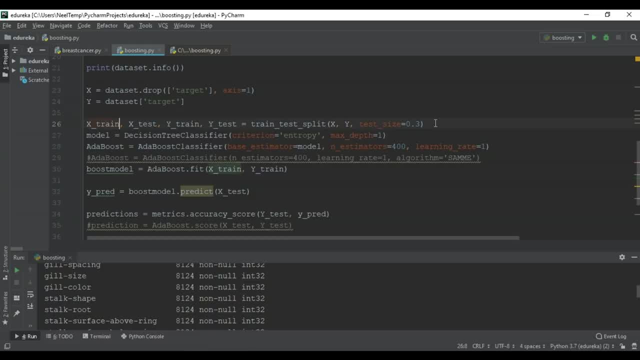 about machine learning if you're studying boosting machine learning. Next, you're performing something known as data splicing, which is basically splitting your data set into your training and testing data set. right, This variable here defines the size of your testing data set. 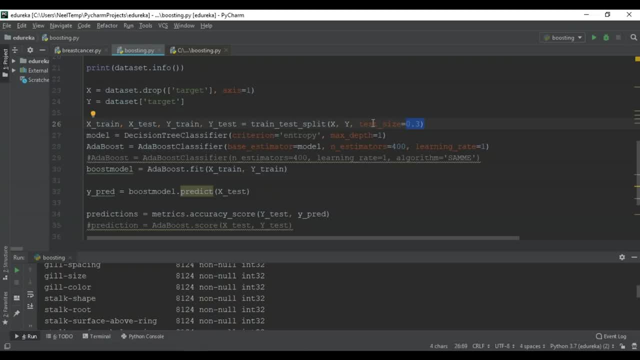 So 30% is assigned for testing and 70% here is assigned for training. After that, we're creating a model by using the decision tree classifier as our base estimator. right Base estimator is basically your weak learner, And here we're using the entropy method. 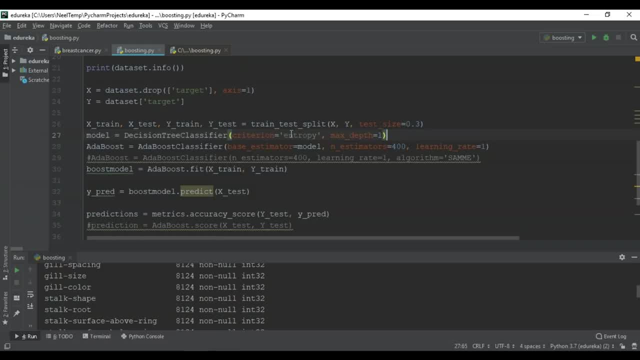 in order to find the best attribute for the root variable. This is a part of decision tree. Next, we're calling this function a DA boost classifier. Now, this is an inbuilt function that will basically do the exact same thing that an adaptive boosting classifier is supposed to do. 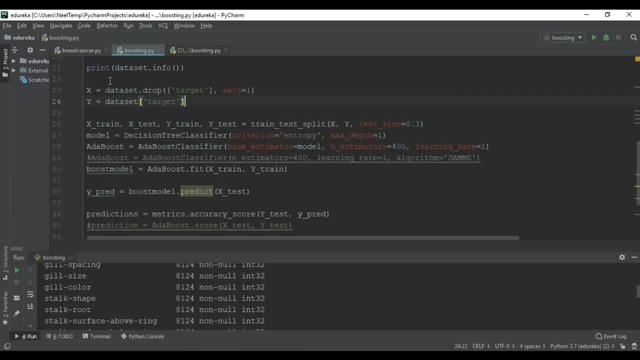 Why is basically created for evaluating your model. So, guys, I hope you all know what all of this is right. I'm not going in-depth into this because this is basic machine learning and I'm hoping that you all have a good idea about machine learning. 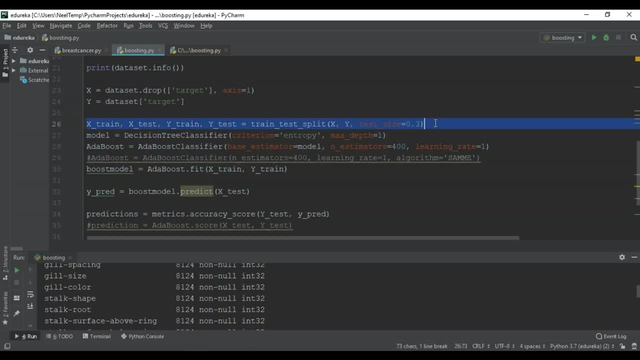 If you're studying boosting machine learning. next, you're performing something known as data splicing, which is basically splitting your data set into your training and testing data set. right, This variable here defines the size of your testing data set, So 30% is assigned for testing. 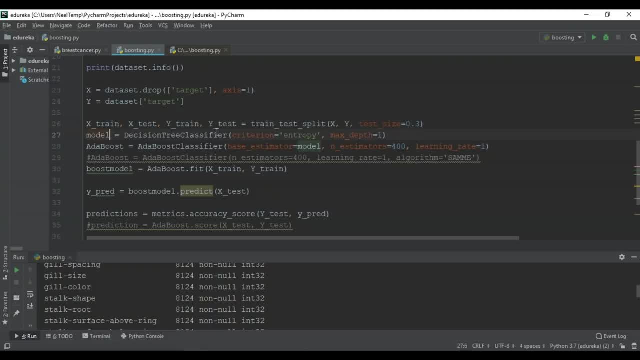 and 70% here is assigned for training. after that, We're creating a model by using the decision tree classifier as our base estimator. right base estimator is basically your weak learner, and here we're using the entropy method in order to find the best attribute for the root variable. 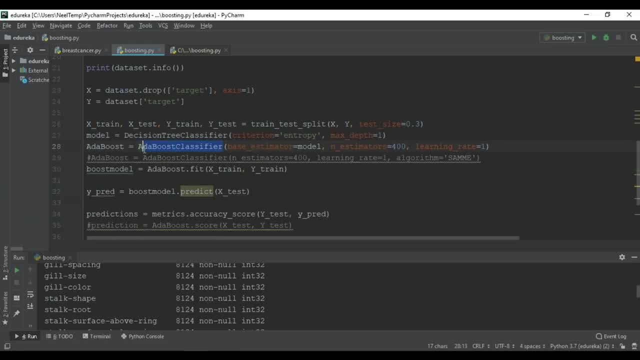 This is a part of decision tree. next for calling this function a da boost classifier. Now, this is an in-built function that will basically do the exact same thing that an adaptive boosting classifier is supposed to do. and the three important parameters that you pass through this function: base estimator. 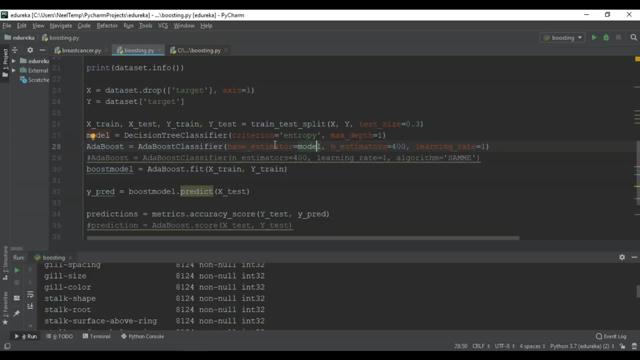 and estimators and learning rate. your base estimator is basically your weak learner, right, and by default the weak learner is always the decision tree, right. So what we're doing is we're just passing the variable model over. here in model, We've stored the decision tree classifier. 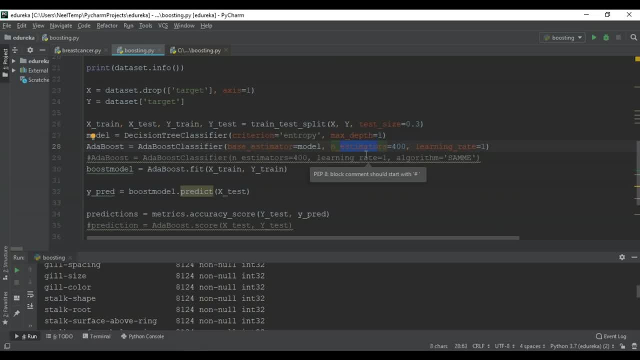 Next, we have n underscore estimators. So this field specifies the number of base learners that we're going to use. right, it just specifies the number of weak learners that we have. in our model, We've assigned a number of 400. then we have learning grade. 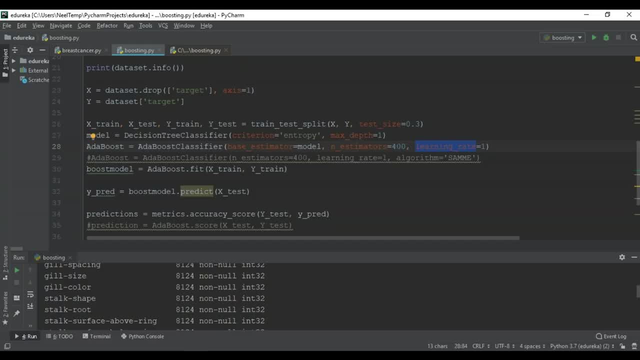 now, learning rate specifies the learning rate, of course, which we have set to the default value as one. Let me just clear that line. That's not needed. next, We're just fitting our training data set into our model. Here we just evaluating our model. 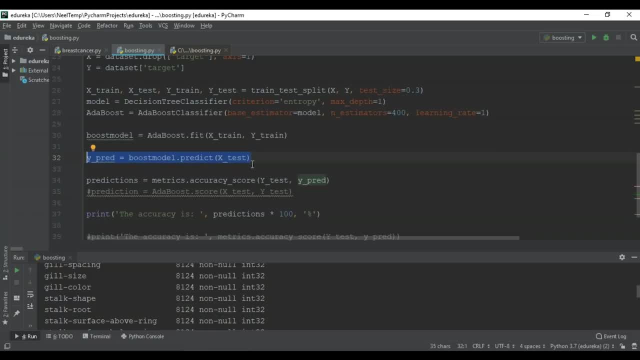 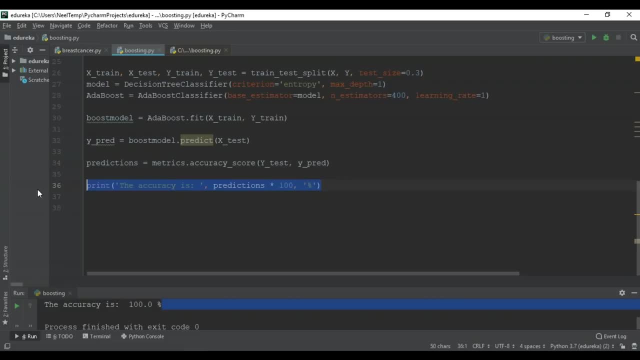 and seeing how it will predict the values when you give it the testing data set. next We're just comparing our predicted values with our actual values. when you do that We get an accuracy of hundred percent. right here You can see the accuracy is hundred percent. 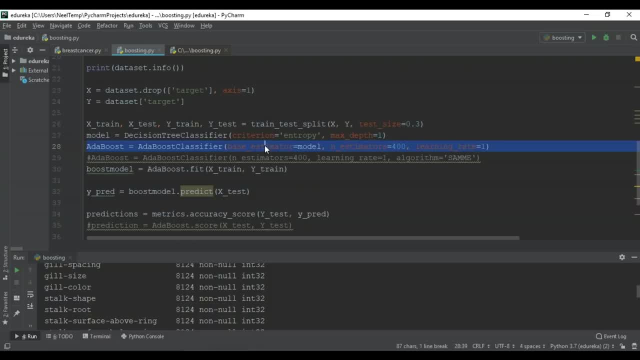 And there are three important parameters that you pass through this function: Base estimator, N estimators and learning rate. Your base estimator is basically your weak learner, right, And by default, the weak learner is always the decision tree, Right. so what we're doing is we're just passing. 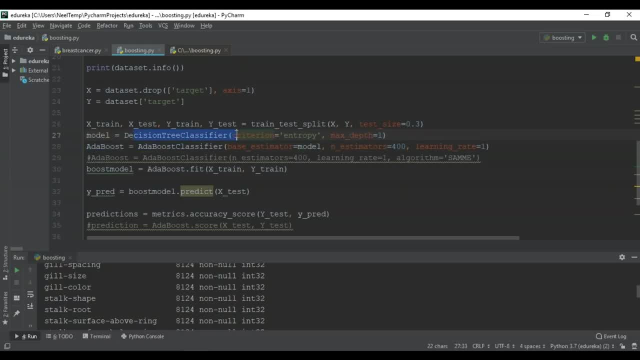 the variable model. over here In model we've stored the decision tree classifier. Next, we have N underscore estimators. So this field specifies the number of base learners that we're going to use. right, It just specifies the number of weak learners. 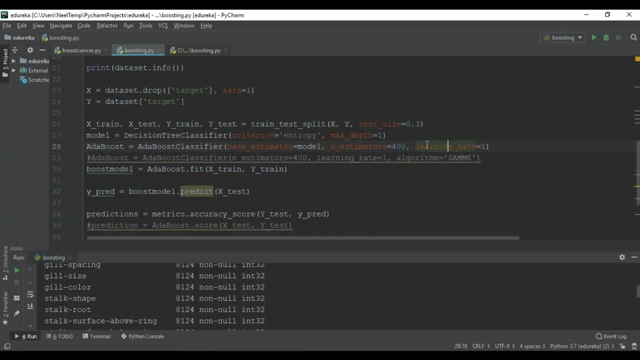 that we have in our model. We've assigned a number of 400.. Then we have learning rate. Now, learning rate specifies the learning rate, of course, which we have set to the default value as one. Let me just clear that line. 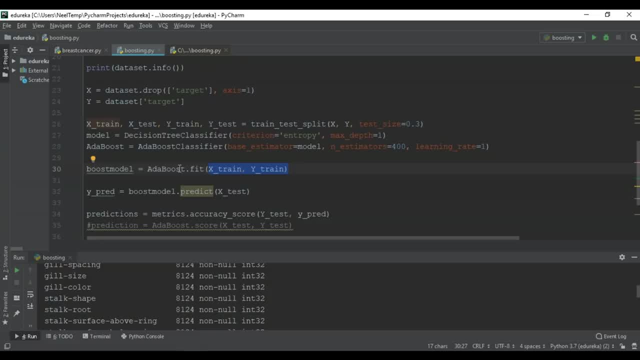 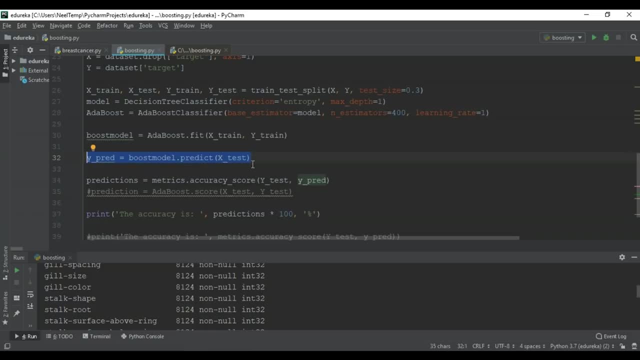 That's not needed. Next, we're just fitting our training data set into our model. Here we're just evaluating our model and seeing how it'll predict the values when you give it the testing data set. Next we're just comparing our predicted values. 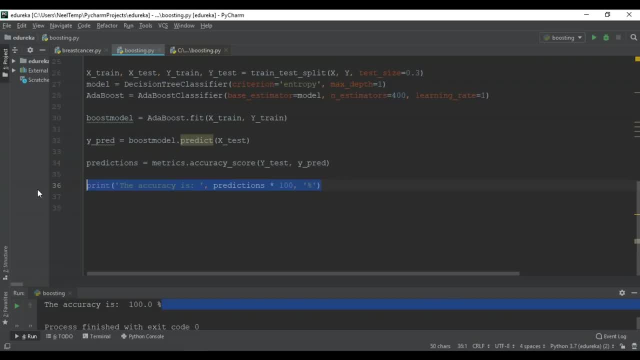 with our actual values. When you do that, we get an accuracy of 100%. Right here you can see. the accuracy is 100%, which is perfect, because this is expected when you use boosting machine learning algorithms. Now, instead of using boosting machine learning, 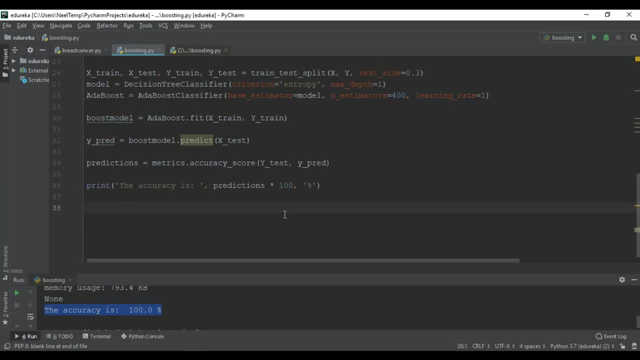 if you try this with just weak learner models like decision trees, then your accuracy will not be 100%. There's always some of the other problem, especially with decision trees- overfitting can occur. So the best way to get your model to increase its accuracy- 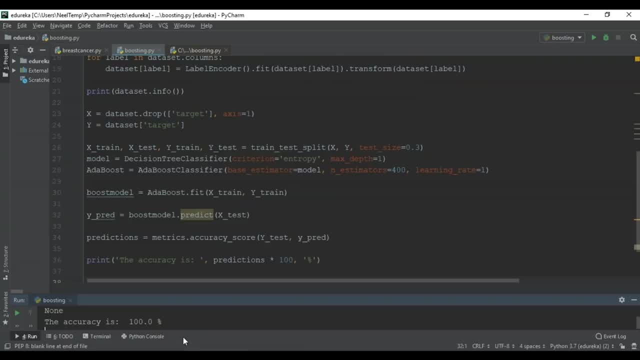 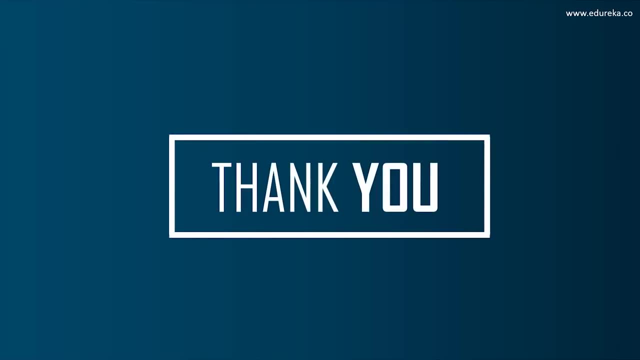 is by using boosting machine learning algorithms. That's exactly what I wanted to prove to y'all: that boosting technique will help you increase the accuracy of your model. So, guys, with that we come to an end of today's session. If you have any doubts regarding this session, 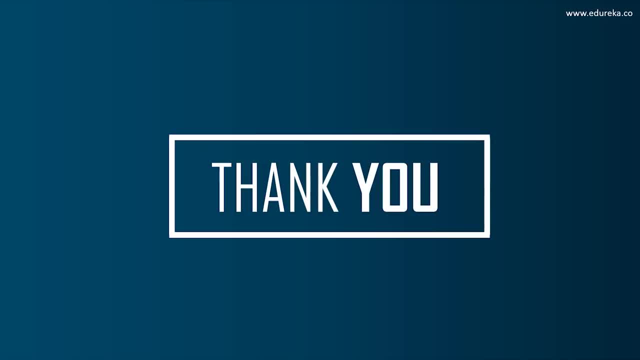 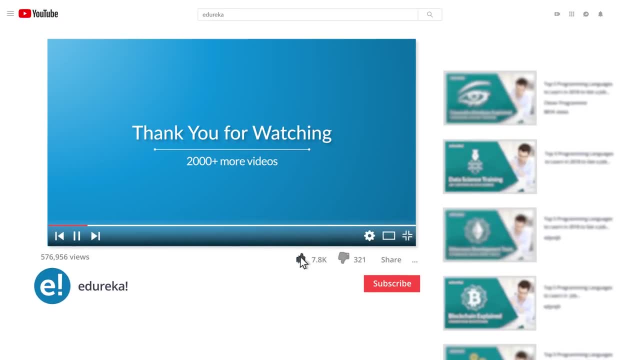 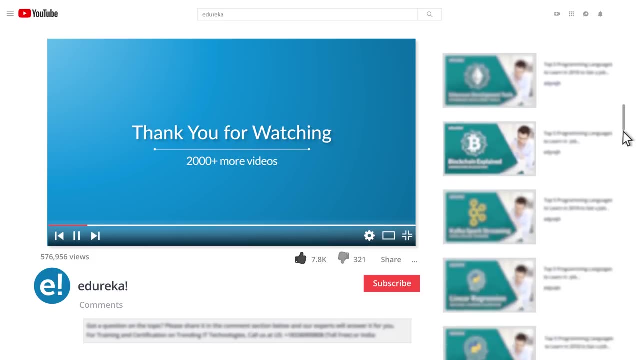 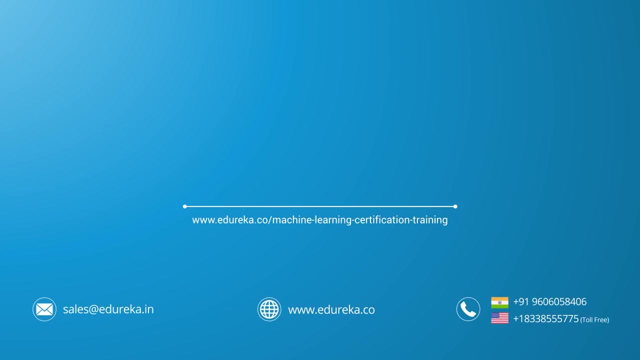 then you can leave them in the comment section. I hope you enjoyed the class and until next time. happy learning, Thank you. 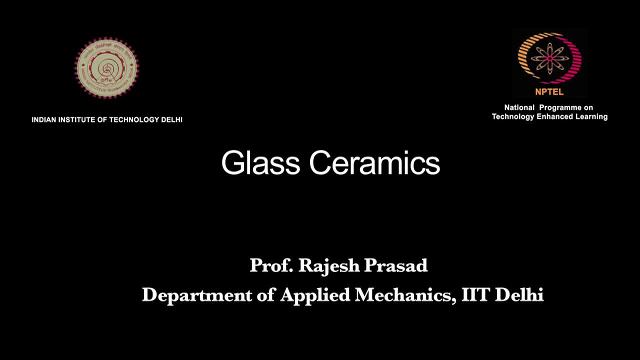 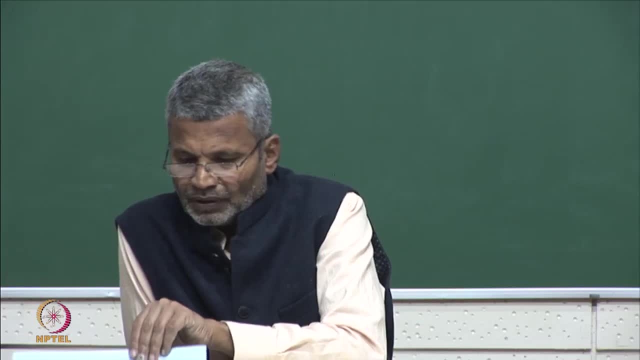 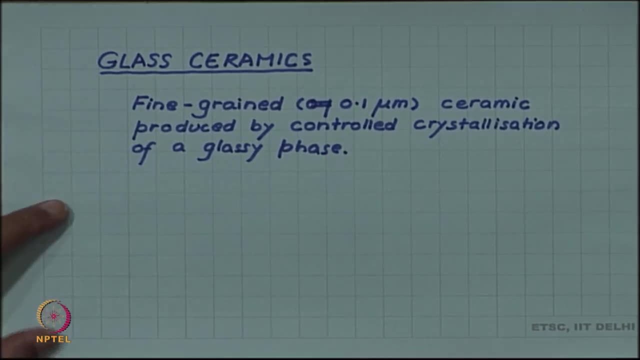 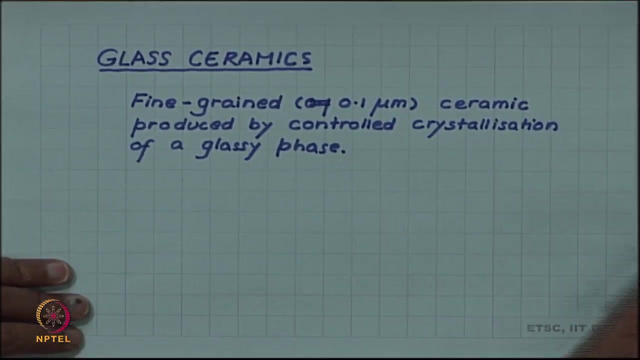 Glass ceramic is an important class of ceramic material which we will now look at. Glass ceramics are actually ceramic materials which are very fine grained- 0.1 micro meter in diameter is the grain size- and they are produced by controlled crystallization of a glassy phase. 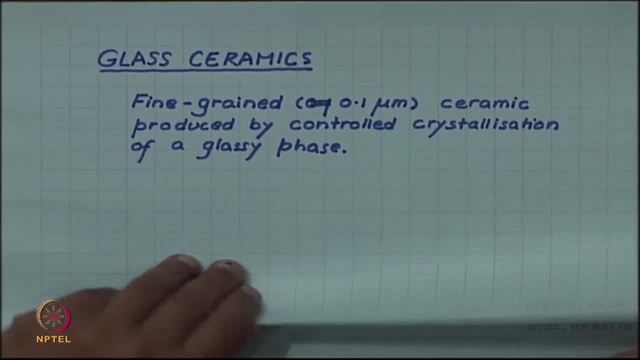 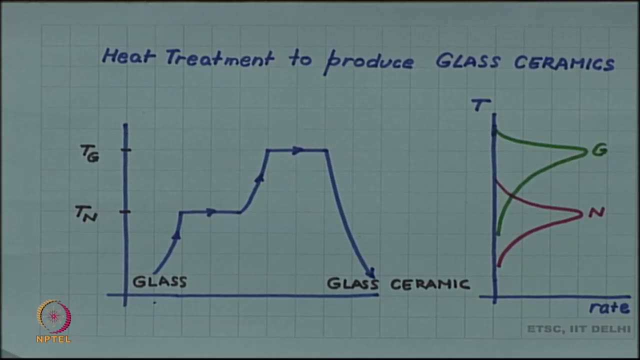 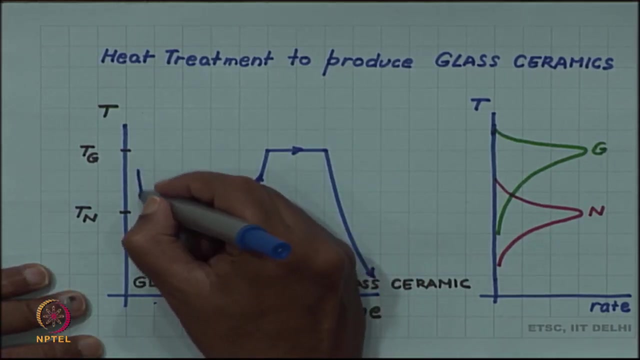 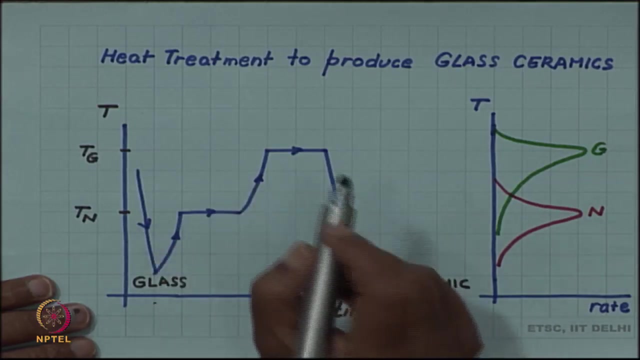 and that is why the name glass ceramic. Let us look at the heat treatment process for glass ceramic. So here is the temperature time. The first figure is the temperature time figure, So it shows the heat treatment cycle. So initially the liquid is quenched to produce glass, Then this glass is held at a temperature at 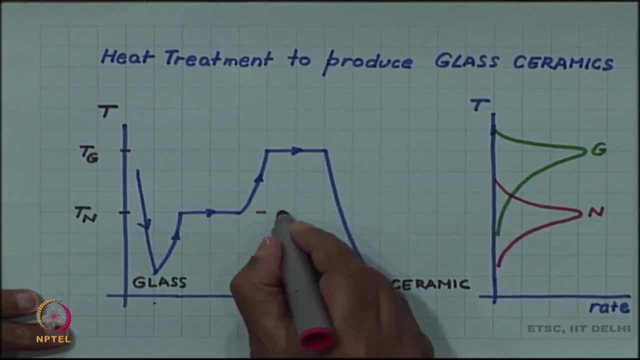 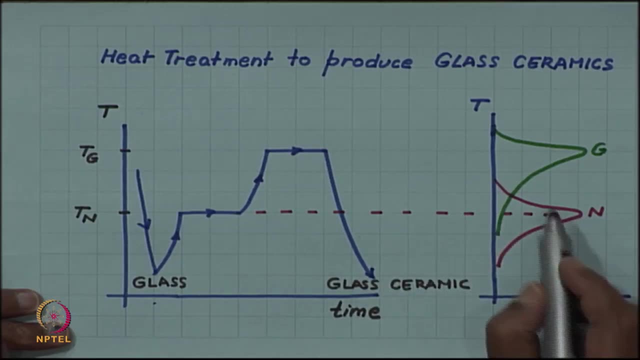 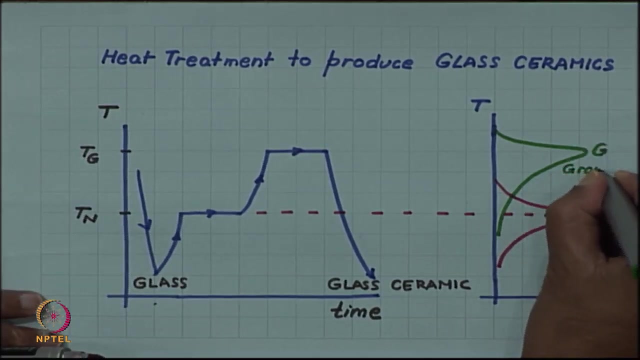 which the nucleation rate is maximum. So this curve. recall we have studied that the growth rate and nucleation rate as a function of temperature, So a maxima. So this n is the nucleation rate and g is the growth rate. So at T, n.